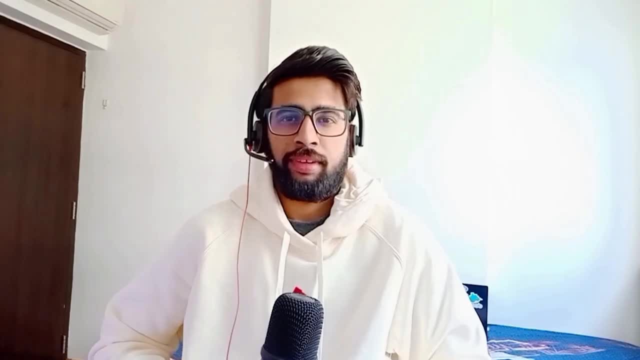 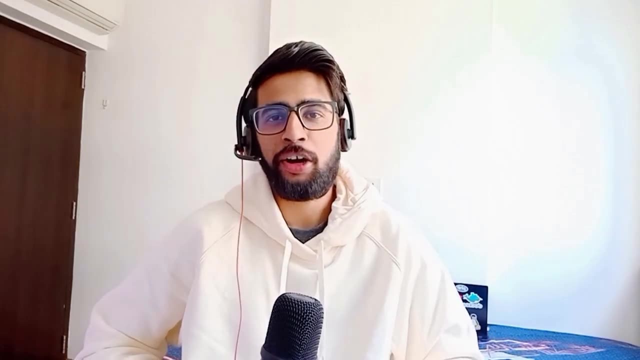 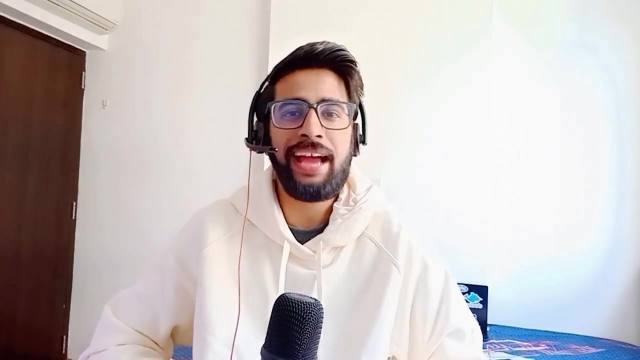 Hello, everyone. Welcome to AI Anytime channel. In this video, we are going to explore that how a small language model, you know, can really perform well, mainly for RAG implementation. And the other aspect of this video will also cover how domain specific embeddings model are better when you compare this with general purpose embeddings model. So we are going to implement a RAG in this video on the smaller models and the domain specific models that you can run it on a compute limited hardware, right? For example, if you have a single GPU, or if you don't have any GPU, you have a CPU machine, and how you can use this smaller LLMs, right? The smaller language model, I'll not call it LLMs now. So the smaller language models, when I say smaller, don't, don't think that it's a 200 million parameters or 300 million parameters. 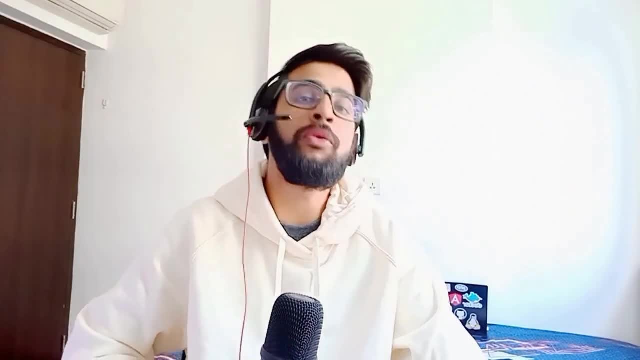 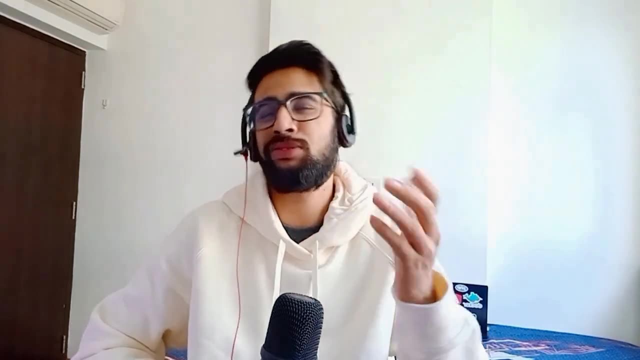 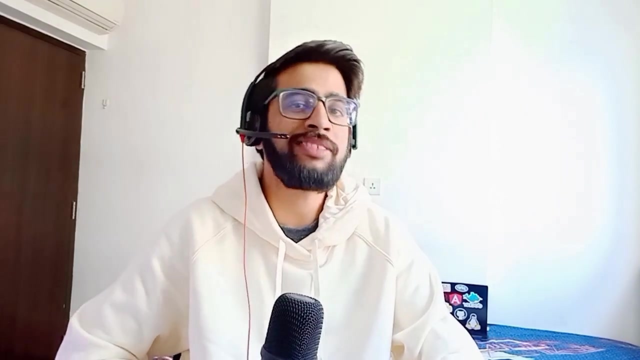 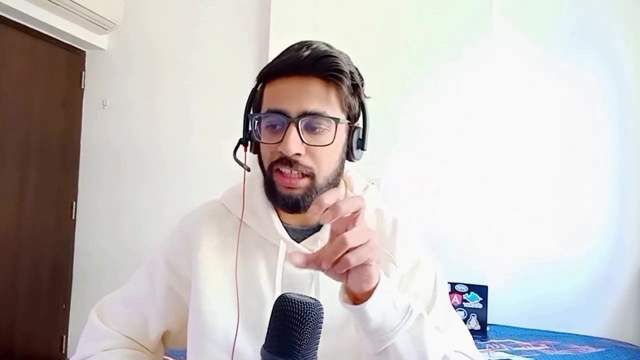 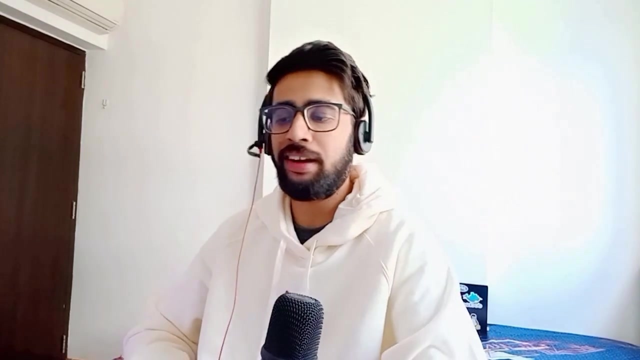 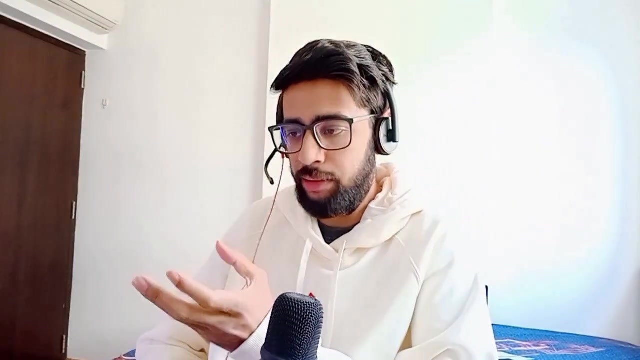 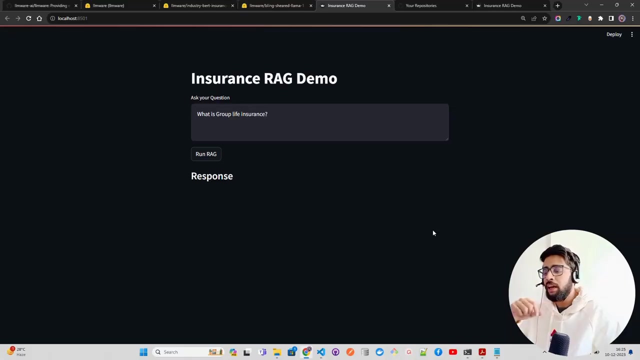 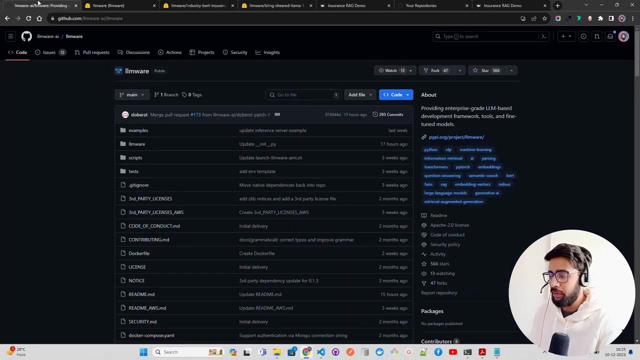 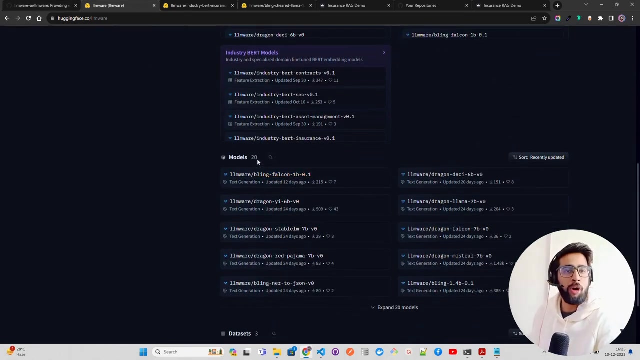 That's not going to work at this moment. But probably 1 billion or 2 billion, right? So its scale has to be on more than 1 billion right now. Language model, which is, which is probably more than 1 million, 1 billion, excuse me, has performed better. And that's what we have seen. But there are some exception, for example, Lamini, you know, with 768 or something has performed better for summarization kind of a task, right? But in this, I'm going to particularly look at LLM where, so if you look at on my screen, this is a demo that we are going to do. This is a demo that we are going to build insurance rag demo. So it's a for insurance industry. And here we are going to use insurance based embedding model that LLM where has created. So LLM where is an organization who has been with contributing really good in the open source community, right? If you look at here on the hugging face, we'll find out LLM where company LLM where AI, they have a GitHub repository as well that I will give the link in description. And they have, they're doing good, by the way, they have 20 models. 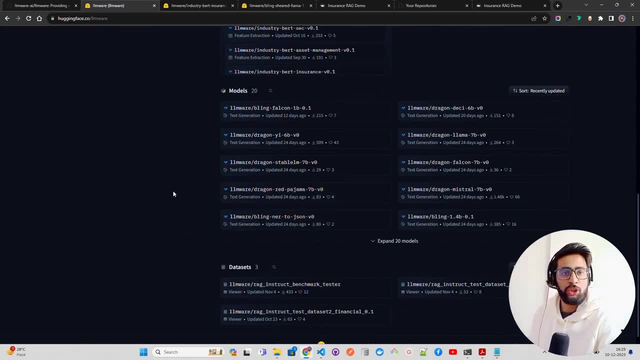 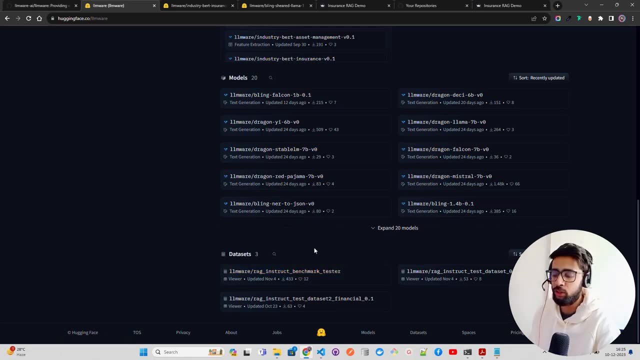 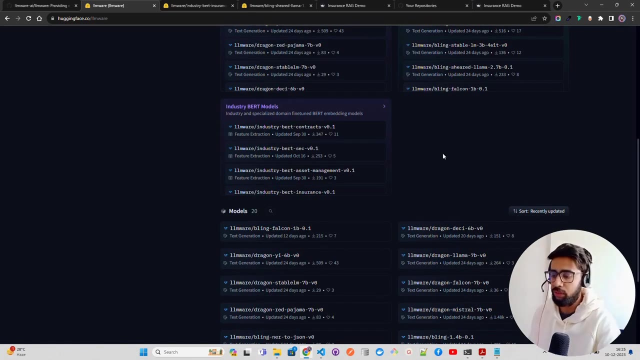 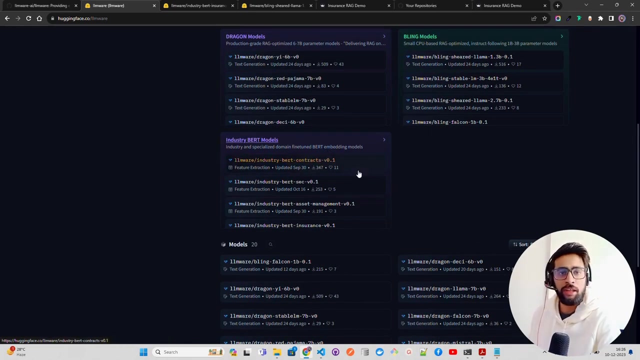 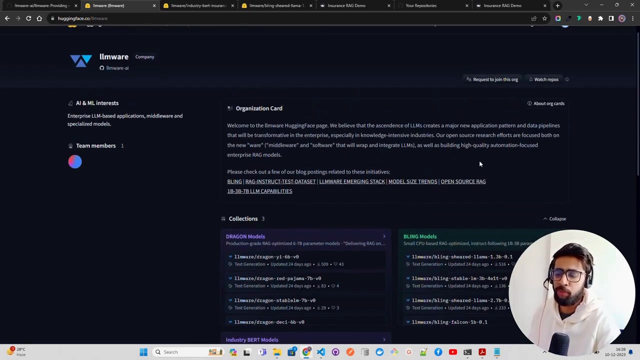 In open source, mostly with Apache 2.0 license, you can commercially use it. And they also have a data set that you can use, right? So they have an instruction rag benchmark data set that you can use to evaluate your other racks that you are building. And some models and some industry specific models as well. For example, you know, if you look at BERT contracts, the BERT based models, by the way, the BERT based embeddings model, that will help you, you know, extract features, which is the first part of your rag implementation. Where you look at the retriever part using an embedding model. Now, they have BERT SEC, they have BERT asset management, they have BERT insurance. Now, you can ask this question that why are we going to use this model? Why not use a general purpose model, right? I think, see, there are trade offs when you work with rag. And I think these are the things that you should know, right? It's easy to build rag, you know, it's very easy, two lines of code, you build rag, right? But when you work for an organization for an enterprise, there are a hell lot of things are involved, cost being involved, etc. 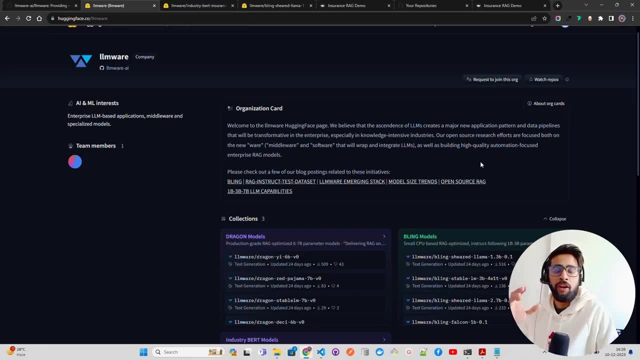 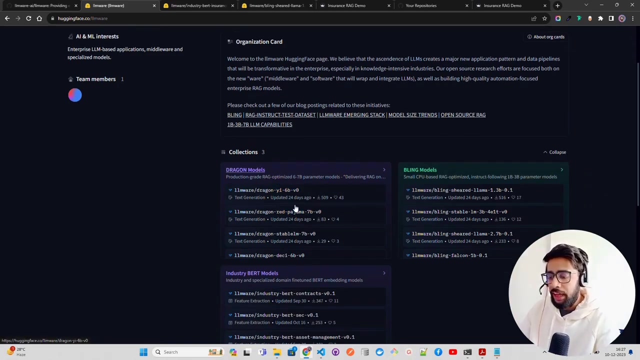 One factor, the security and compliance being the other factors, not everybody will use closed source model, a few of the organization will like to use open source, everything on premise within their infrastructure and network. So if you work for those kind of organization, this video is helpful. If you work for like some hobby projects, pet projects, you know, then you don't watch this video, I recommend don't waste your time watching this video of mine, right? So this video is important to understand that what are the requirement when you work for an enterprise that you have to look at, don't only how many specific model that will help, you know, build better retriever, then you would use smaller models that is very particular, that will be used particularly for a use case, you know, very specific use case, like, you know, asset management or underwriting the risk, etc. Right. So these are the things that I'm going to cover in this video. And if you look at here, they have dragon models, LLM, where dragon rate pizama dragon, you know, stable LM language model 7b. So these are the 7b models. One is a six 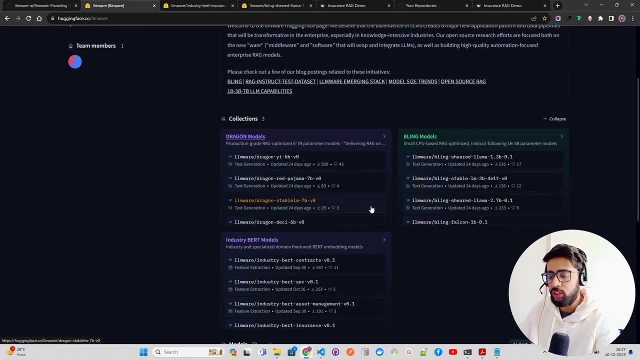 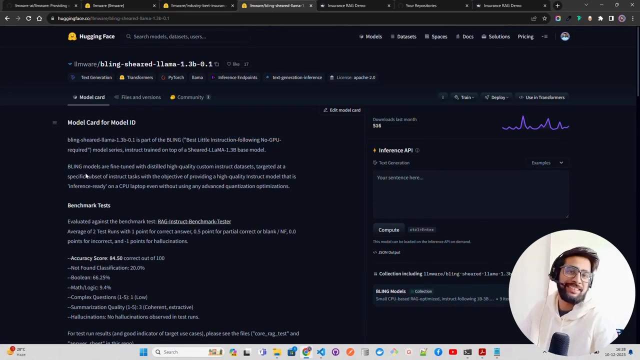 b model and the other is a dashi 6b version zero right so this is a dragon model then they have bling models and i'm going to cover bling i'm going to cover this lama seared sharded model i'm not sure what seared means by the way but sharded i understand okay so bling i think which is an acronym for i don't know i forgot the acronym there's something related to best little instruction following no gpu required which is which is really intuitive and funny as well right best little instruction following no gpu required so it says that you don't need gpu to inference this model or use this model right this is what we're going to look at here let me just ask this 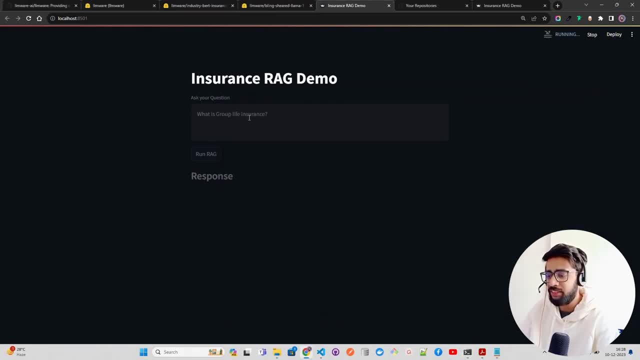 question but i don't know after running it let me see if i'm running it yes i'm running it i've asked a question what is group life insurance and you can see it says generating response and you 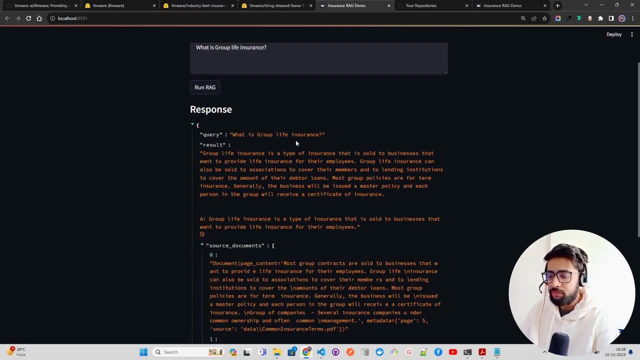 can see i got my answer uh this was your query what is group life insurance and then you say okay group life insurance is a type of insurance you know that is sold to businesses you know that is sold to businesses and then you say okay group life insurance is a type of 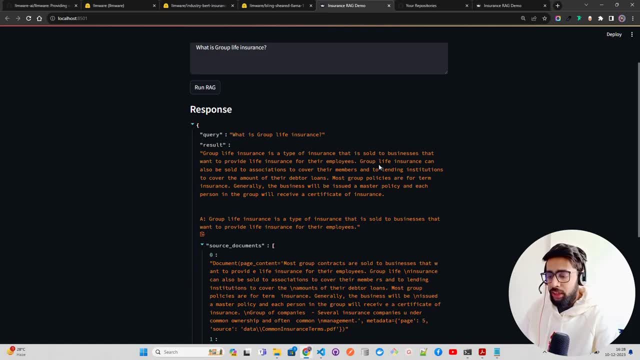 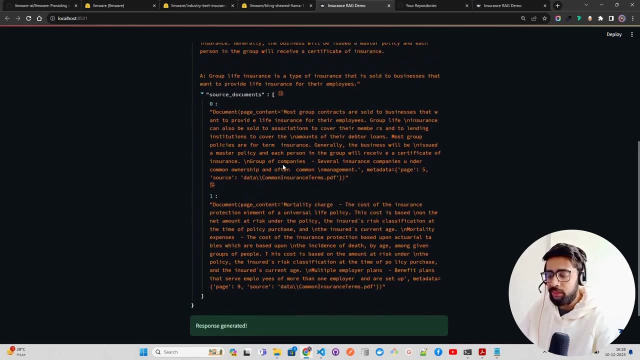 uh that want to provide life insurance for their employees group life insurance can also be sold to association blah blah blah and then we have top two documents uh as uh top k which is 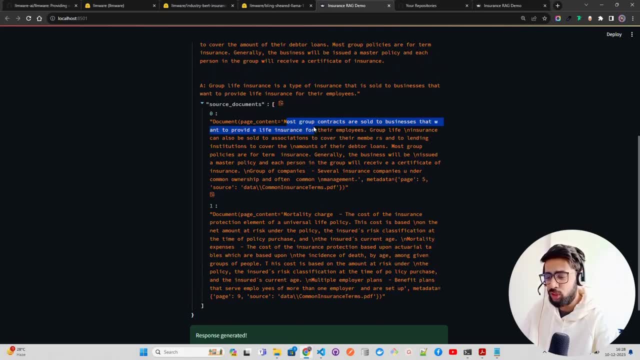 equals to and you can see it gets it right right most most group contracts and group life insurance can be hold and this is the document by the way guys we are using so we're going to use this 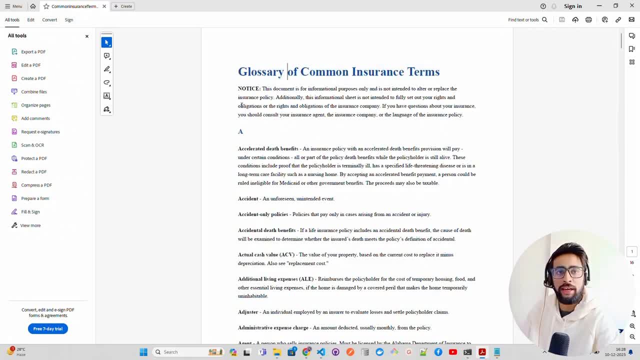 document to as a source document and you're going to create a vector store out of this and you can see it says 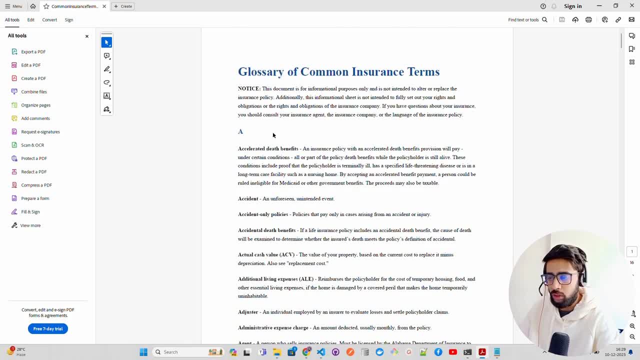 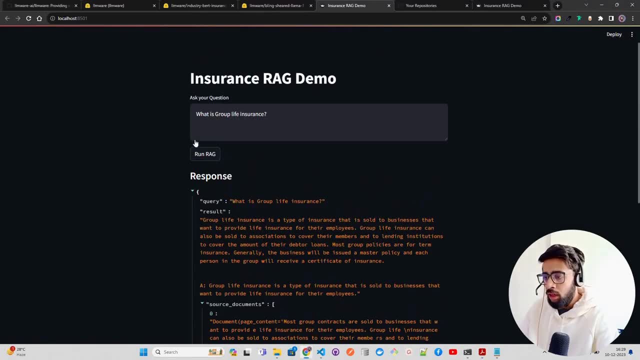 glossary of common insurance terms okay now this is like our terms terminologies of insurance terminologies that we use right this is what it is we're going to cover this 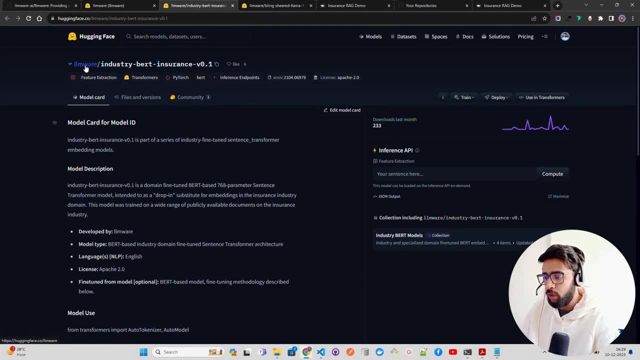 embedding model industry bird insurance okay it's by llm where again you can see what they say it says it's a part of series of industry fine-tuned sentence transformer embedding model it says 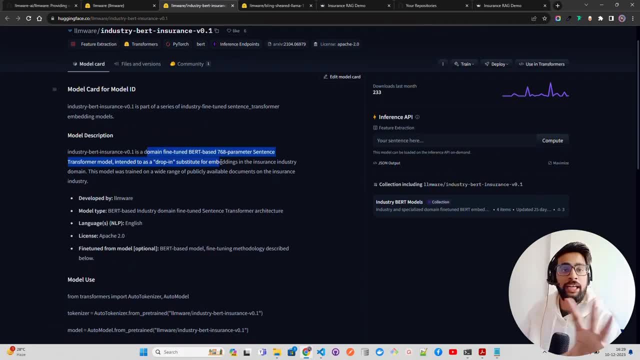 a domain fine-tuned i already have covered in my meditron video i'll give the link in description where i have the link in the description and i'll give the link in the description where i have the 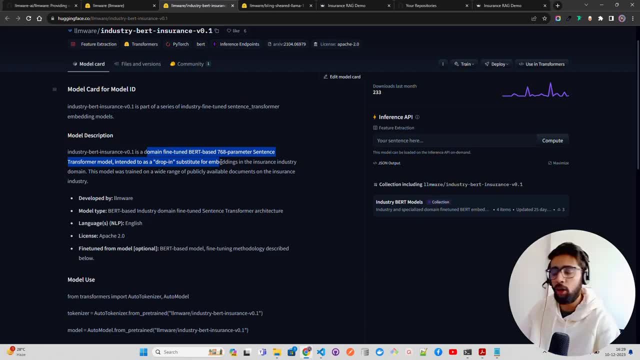 use pubmate but right which is a medical embedding model and it performed better than general purpose model and they are smaller in size as well now you see it says a domain fine-tuned birth base 768 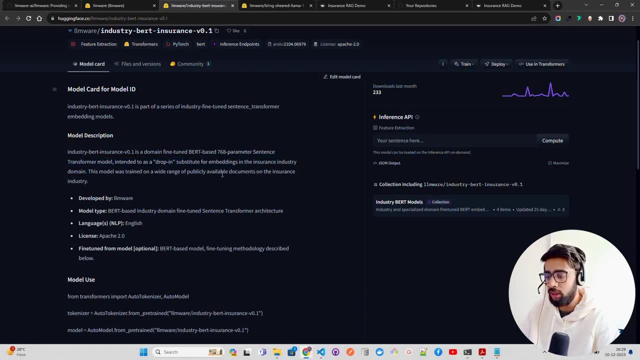 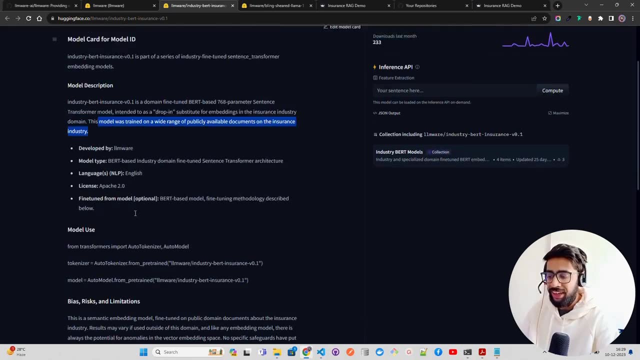 dimensions as a 768 parameter sentence transformer model intended to as a drop-in substitute for embeddings in the insurance industry domain fantastic right it's available documents on 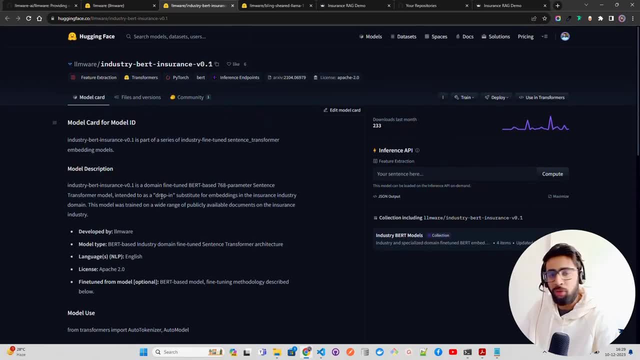 the industry insurance industry when you work with deep learning or natural language right it is it's all boils down to weights right when you use when you fine-tune this model you know on particular 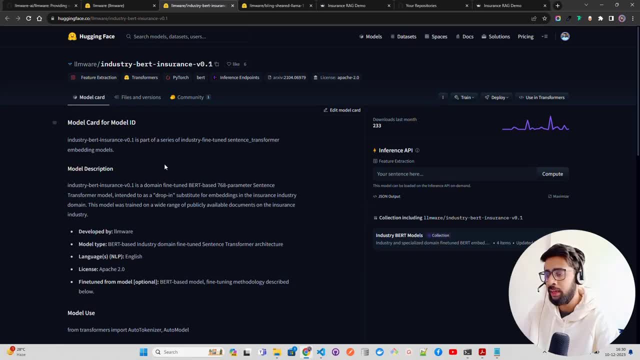 databases like insurance in a domain or industry the model understands the taxonomy better than a general purpose model if the general purpose model has lesser corpus when you compare with a domain 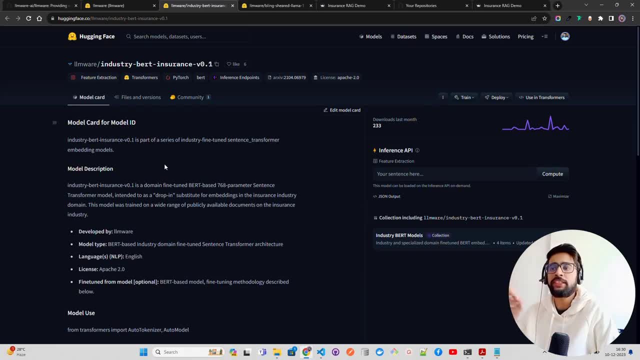 specific model and that is why it's very important because it all boils down to weights the weights there is some weights assigned to these keywords which is more domain specific and once you use 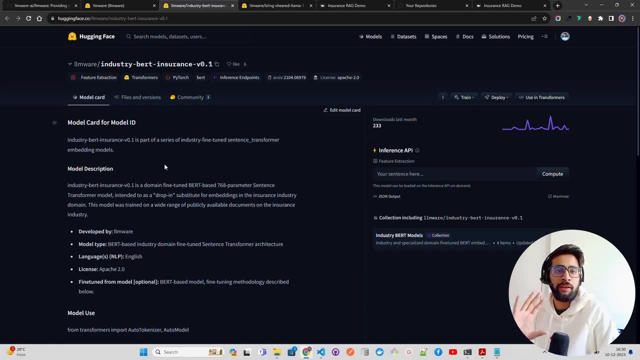 this in your similar use cases the vectors will be very similar okay they will understand the model will understand okay the search has been uh the search has been you know uh they've been 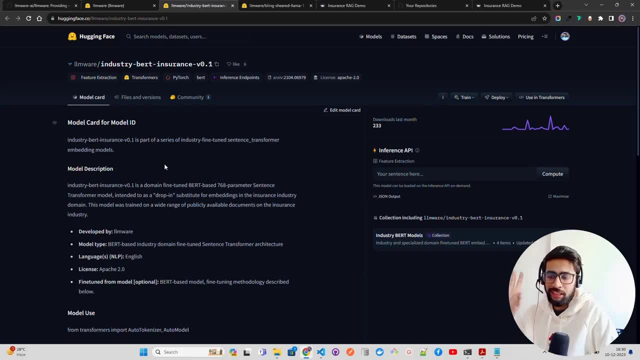 done on this vector so let me return a similar vectors right so this is very important now let's 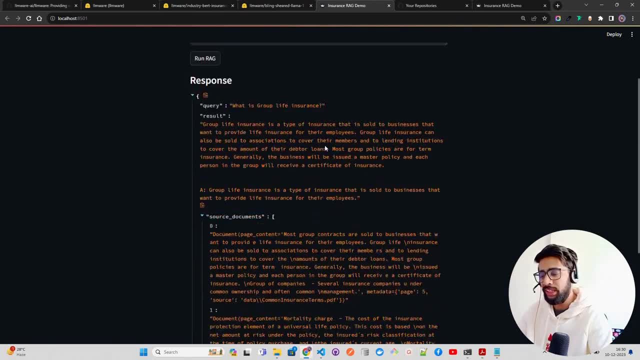 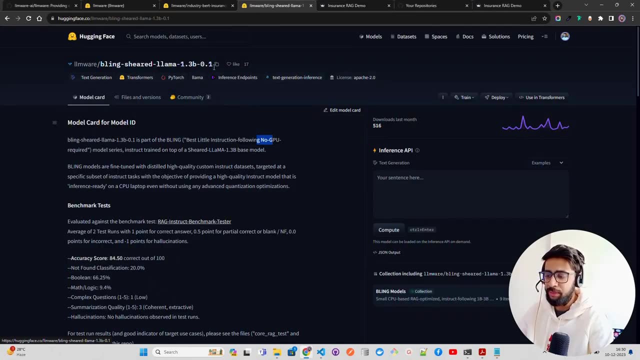 start uh building this app insurance rag demo that you see is going to go build a streamlit application uh using lmware model you can see it's a 1.3 billion model of llama and 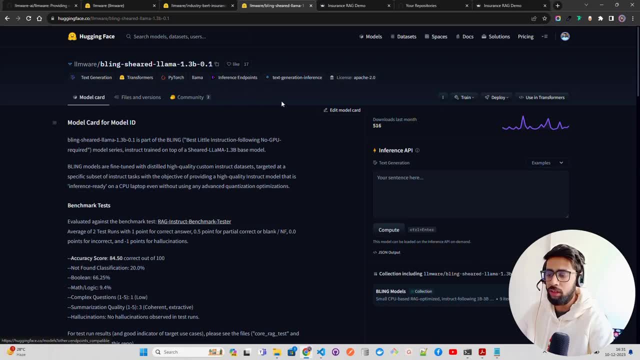 we have llama 7 billion and you can find out this is fantastic right more than 80 percent right size reduction so 80 percent of lesser size when it comes to the params as well and also with the compute memory right and that's why you can you can easily deploy it and even you can inference 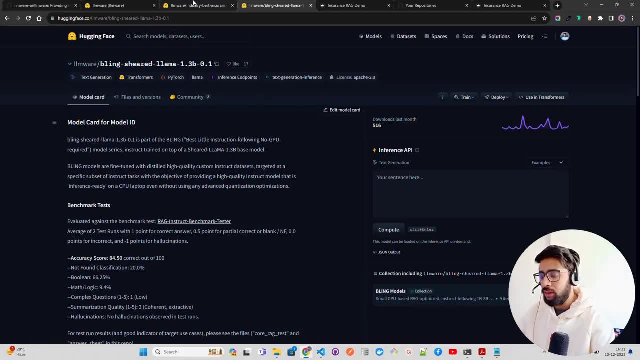 your own cpu machine so let's start building this we'll combine both the lmware models today one is for uh embedding model of the bird insurance and the other one is the lmware model of the 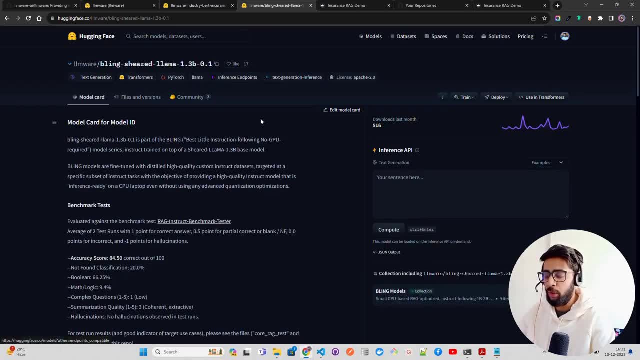 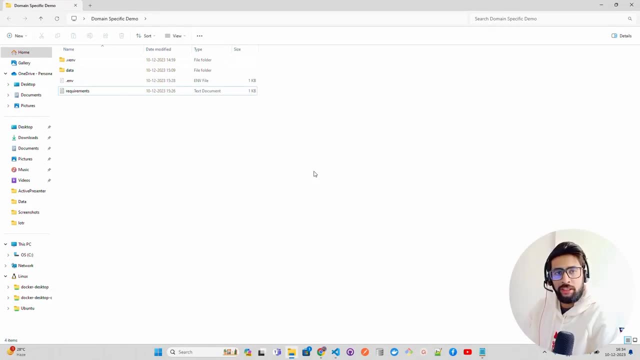 blinks seared llama 1.3 let's start building this guys all right so to build this uh application the rag implementation that we're going to do with lmware embedding models and the lm what we're going 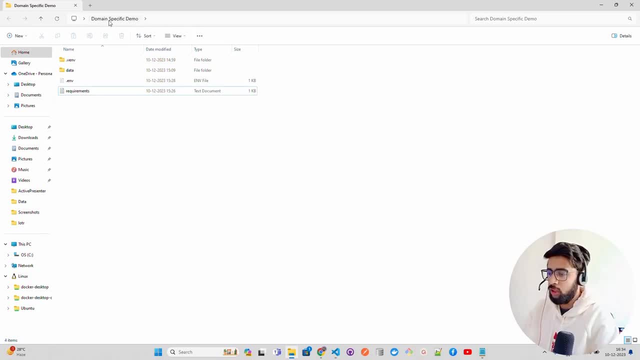 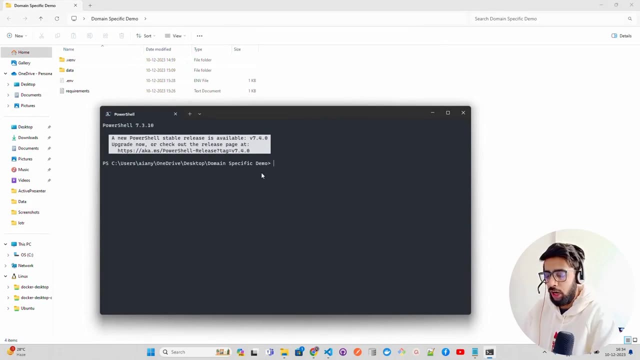 to do is create a folder first you can see i have something called domain specific demo i'm going to open this in terminal and you can see i already have a virtual environment i will show you how i created it if you don't have if you have an account you can use that and if you want to create you can 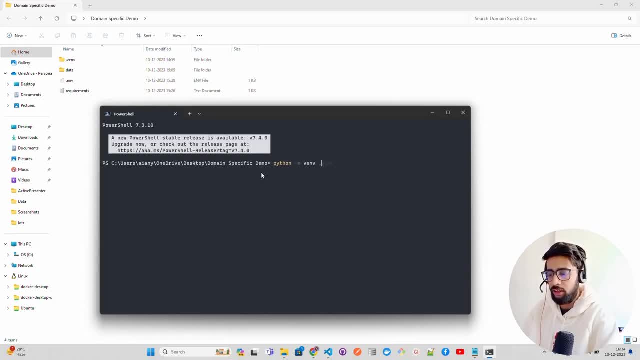 use python hyphen m venv dot venv and you hit enter and it will create a venv for you you can use some other ways of creating as well using virtual env as well right so that's how you do it 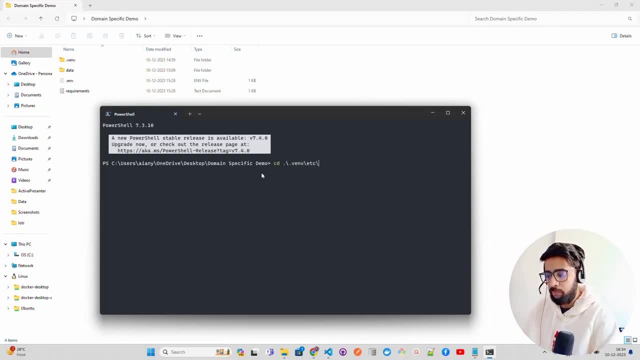 let me activate this is how we activate on power cell scripts and then dot slash activate if you are on linux you have to do go to bin not scripts and then you do source activate uh let me just do 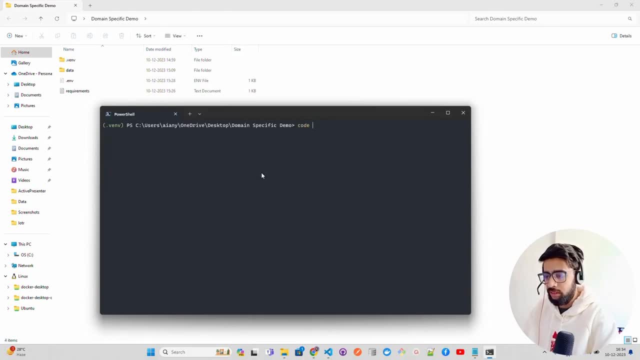 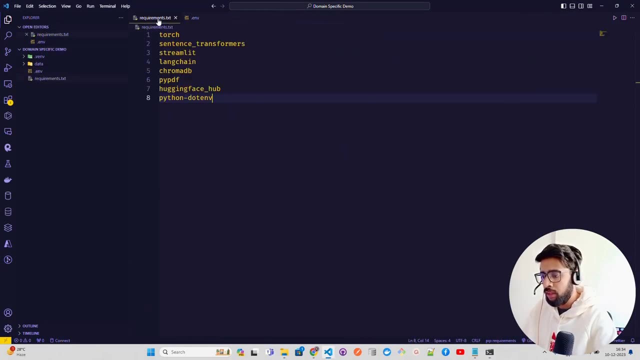 couple of three dot dot clean this and open this in vs code once i open this in vs code i'll explain a few things here uh and by the way i'm you can see that i'm using hugging face api token of course 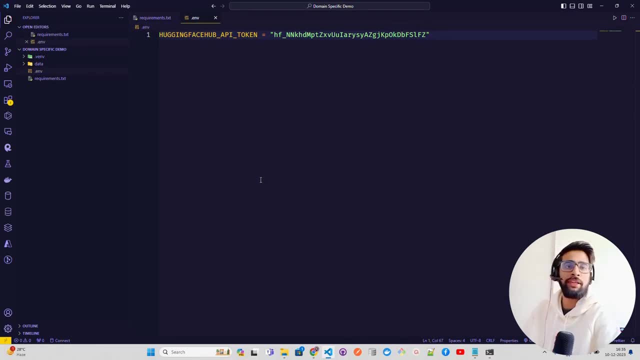 i will delete this after the video the reason is i'm using the inference api from hugging face to use the language model i'll show that in a bit but let me first create something called ingest dot 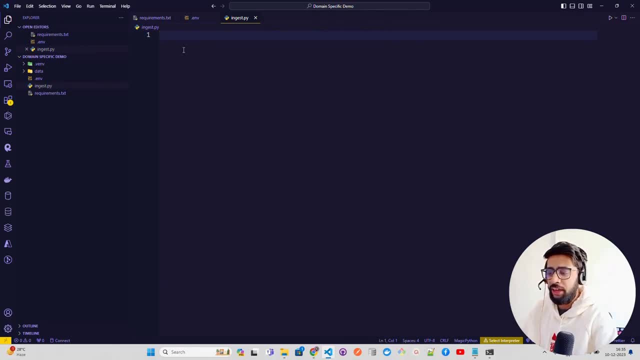 pi now once i create ingest dot pi here i will write all the code for uh creating the vector store uh using an embedding model which is the domain specific embedding model of lmware now you 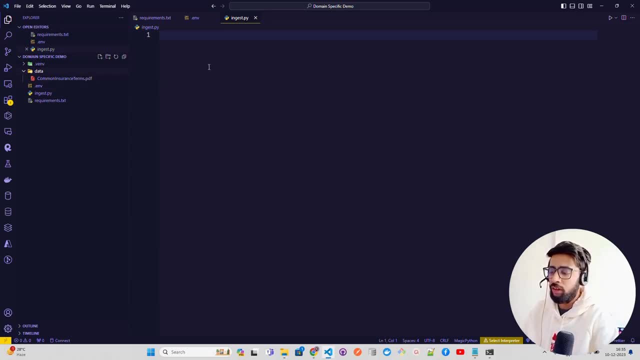 can look at i have a one single file you can keep multiple files depending on if you want to if you have you know like if your document store is too big your database is too big then you probably 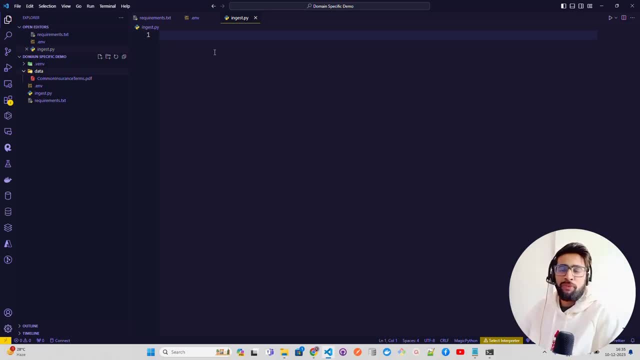 need a vector database not a vector store chroma dv files is like they're not that good when it comes to build uh you know implementing solutions at scale okay you have to look at wav 8 qdrant 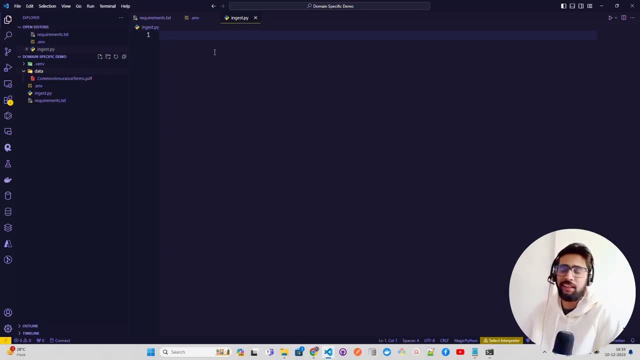 milwa spine cone and uh etc right there are a lot of others now in the ingest dot pi the first thing 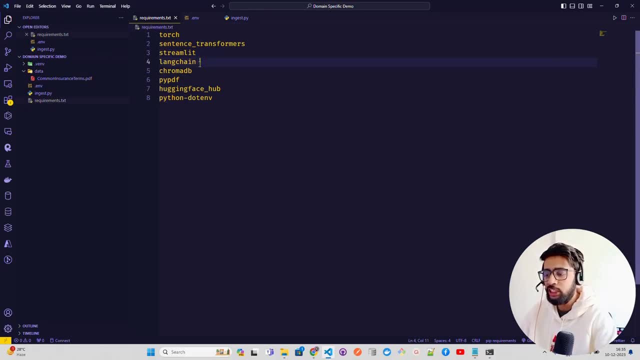 we're gonna go ahead and build is Notes sentence transformers St 혼le torch sentence transformers st Hait lang chain chroma db pie pdf hugging face hub and python.env this will be available on my 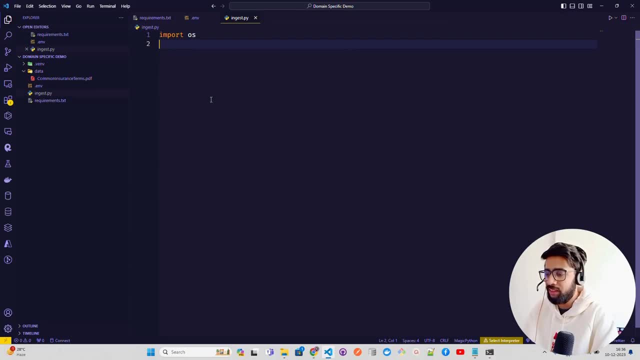 github repository so you don't have to worry about it now the next thing is on ingest.pilot let me just do few things uh import OS i don't know if i need it then from langchain.techsplitterimport recursive character text splitter i'm going to use recursive character 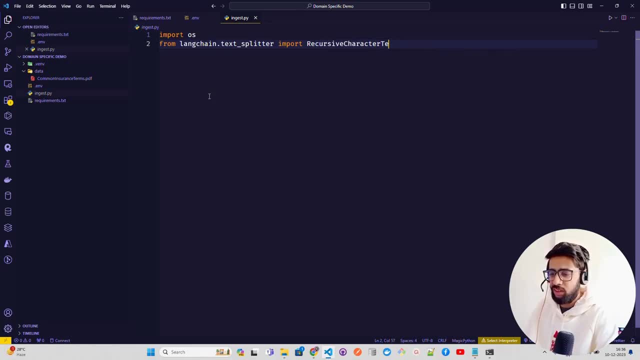 uh text splitter or whatever okay uh let me just do that and the next is document loader i need a document loader so from langchain dot a document loader because i have my data in a directory so 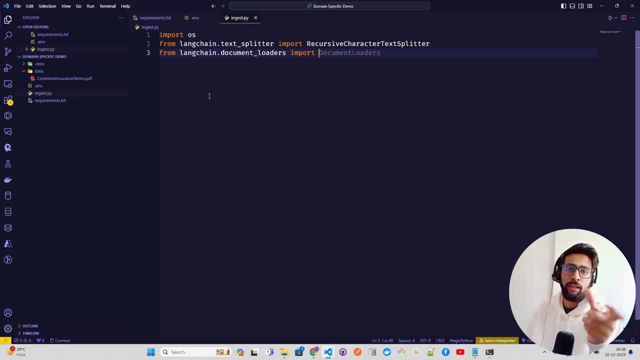 just go to my rag playlist i have more than 25 videos on rag go through all of the videos and you'll be a rag expert okay so uh import directory loader uh directory loaders okay 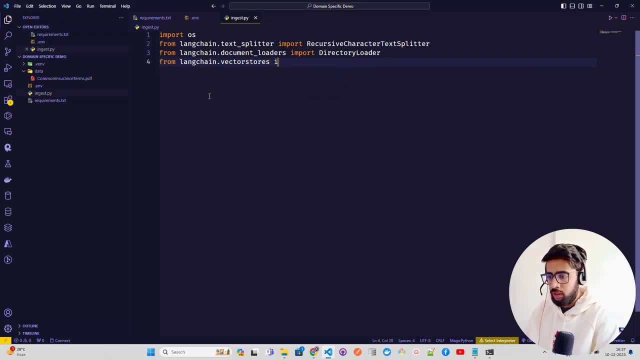 uh import what i'm going to do is import chroma from langchain dot embeddings right so for that i'm going to have now here i'm not going to use hugging face 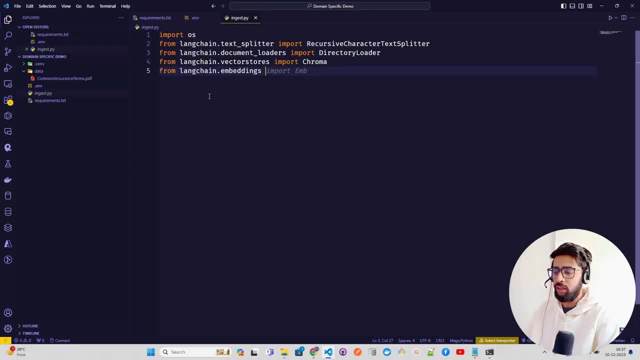 embedding i'm going to use sentence transformer embeddings i'm going to use this embedding model through sentence transformer so let's do that so for that i'm going to do 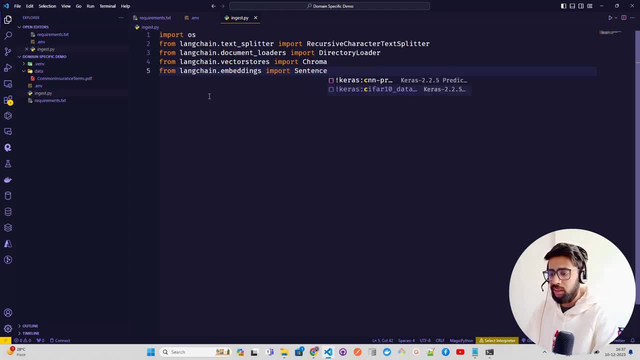 import a sentence uh sentence transformer embeddings this is what i'm going to do 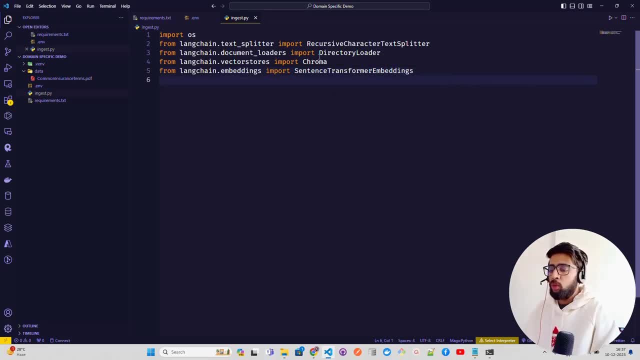 fine now the vector store chroma is done the document loader directory loader is done 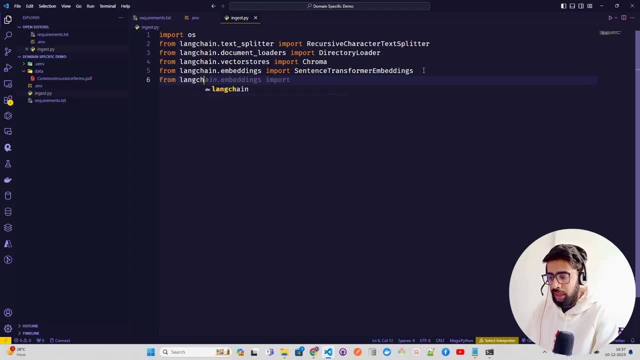 and then we need pi pdf guys there's a pdf file so from langchain dot uh again right for that also document loaders let me just get it after directory 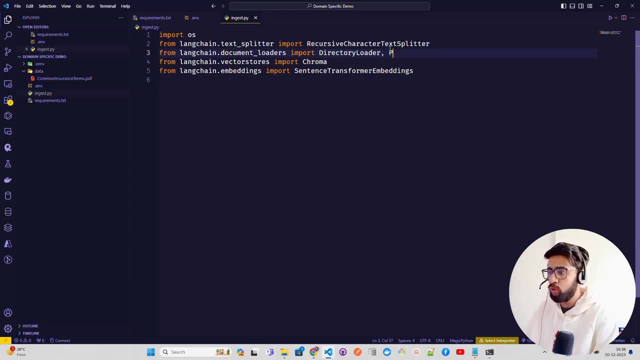 loader only okay not no need to write something new right here i'm going to use pi pdf loader let me just do a print and see if i am able to load it successfully load it 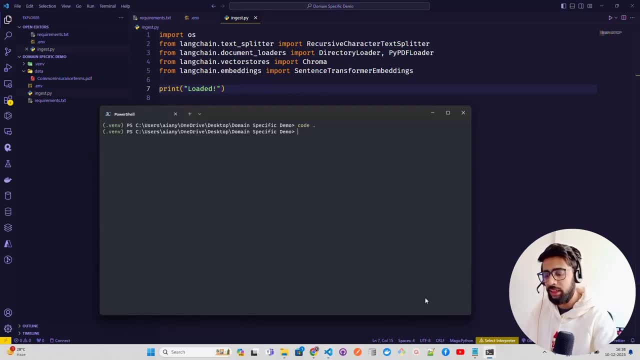 something like this okay this print message gets printed in this make uh you have done it right it's an english dot pi loaded right let's remove that our import is successful now the next thing 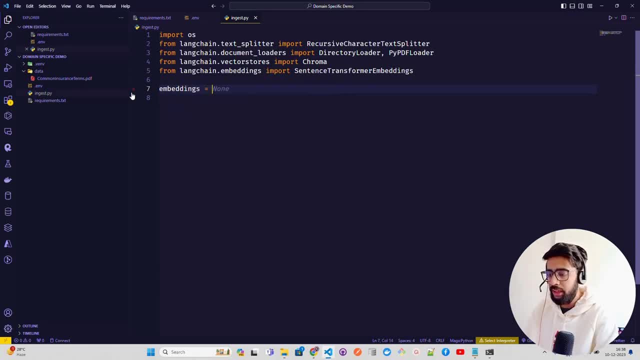 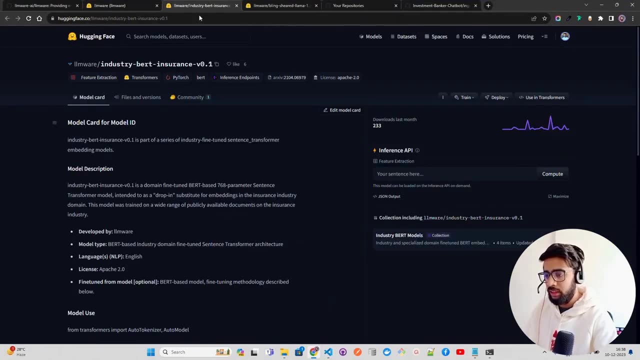 is to have this embedding model so let me just do that embeddings equals and i'm going to use sentence transformer embeddings and in this you have to pass your this thingy uh this hugging 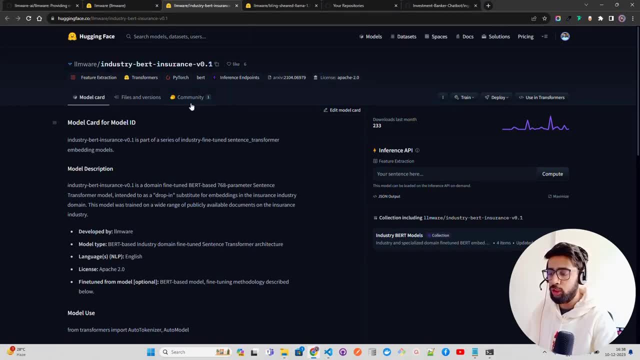 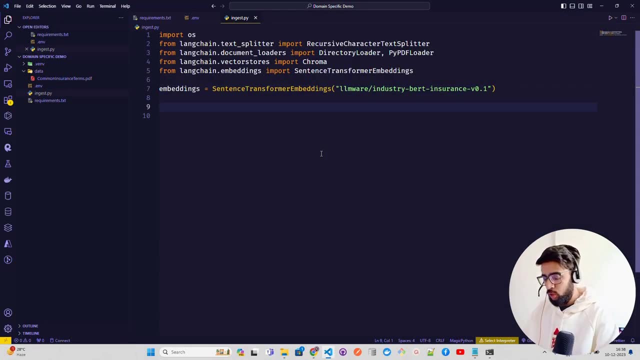 face link you know of the embedding model the insurance is domain specific embedding model let's do it here and then you have your embeddings 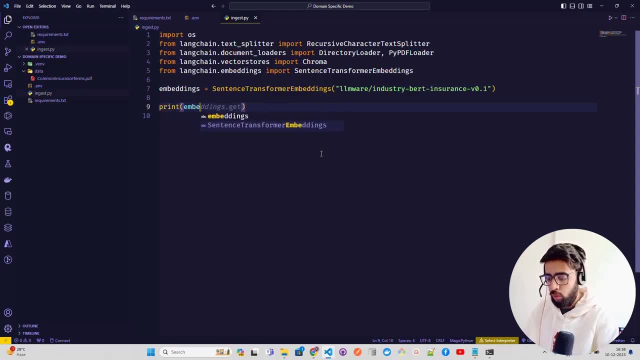 thingy done now let's just print the embeddings if you want to look at the pipeline of this embedding model okay now print embeddings the next day is we need a loader variable to load 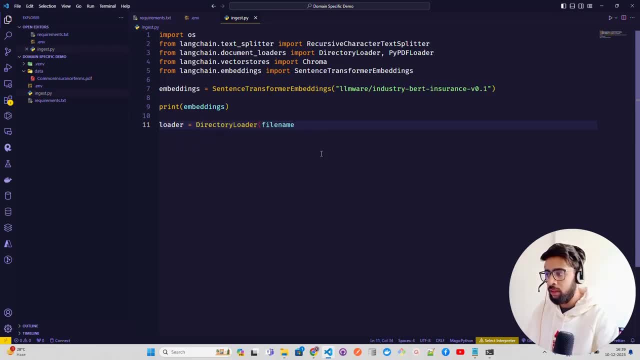 the file so directory loader thing and then i have my folder as a data data and i will just close the data okay now data and then i'm looking at globe and globe is like i have to define a pdf thingy here so where are a couple of stars and then uh dot pdf thingy and then i have my folder 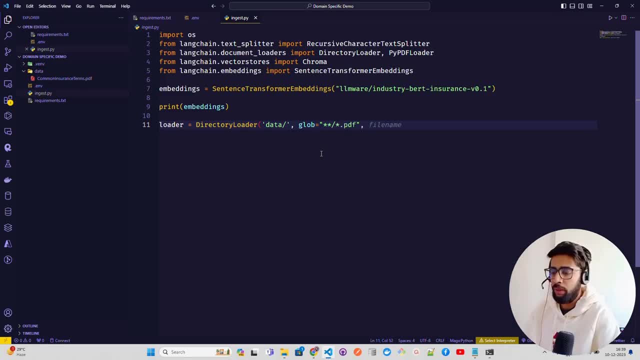 pdf if you have csv if you have word you have doc x doc whatever you have to define like that that's a better way of doing it let's do so progress to track this in terminal so so progress 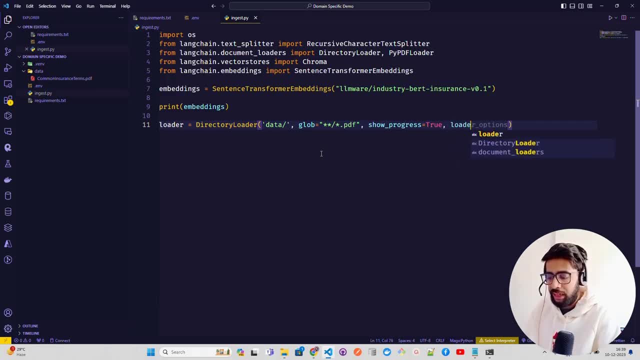 equals to true and then i'm gonna have a loader class i want the directory loader thing to use pi pdf library to know extract the uh load and extract the data so the loader cls and the excuse 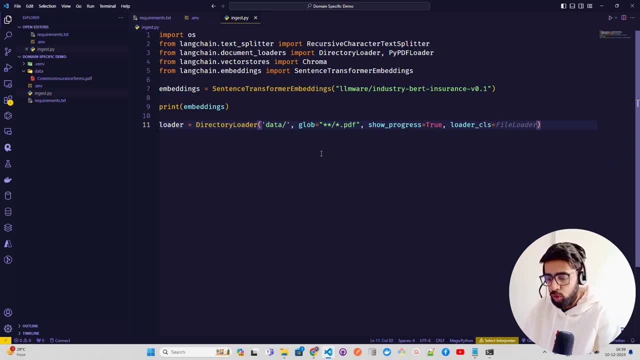 me this underscore loader cls equals that becomes your pi pdf thingy so pi pdf loader you can also use pi pdf itself it's fine loader is done now let's use the documents 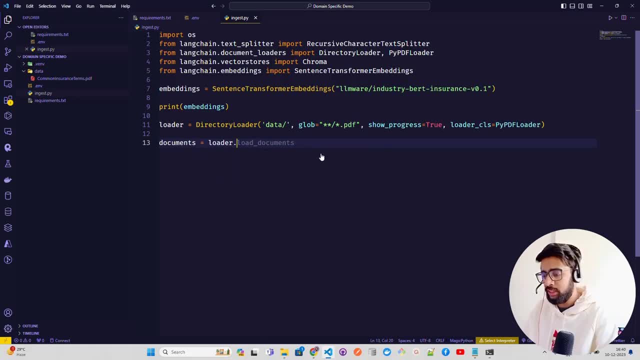 variable pretty much you go on lanchan documentation you'll find this loaded out load once you load it out load you are done you have to define a text printer with some chunking 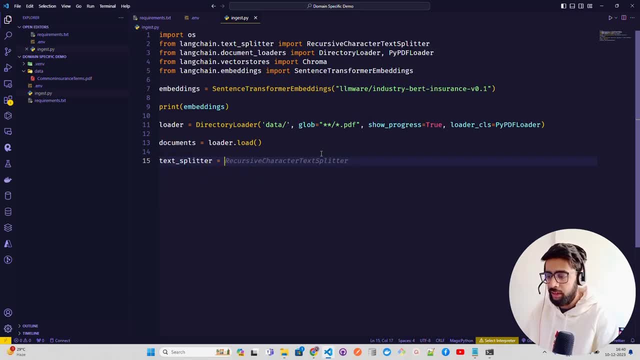 strategies very simple chunking strategies it's like trial and error you have to keep trying it and see which chunking strategies work good for you now chunking uh not not 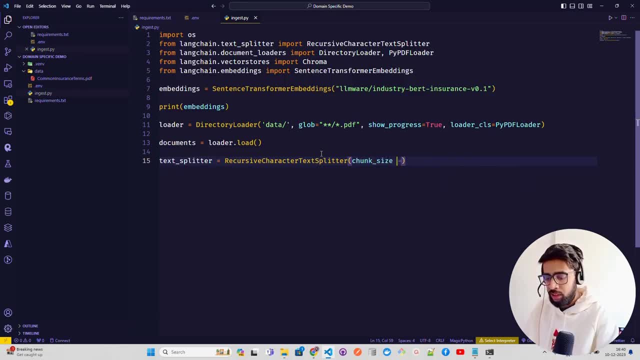 chunking uh chunk size chunk size let's keep it around i don't know maybe 700 okay and chunk overlap for how many chunks it should overlap let's keep it 70 one tenth i always keep one 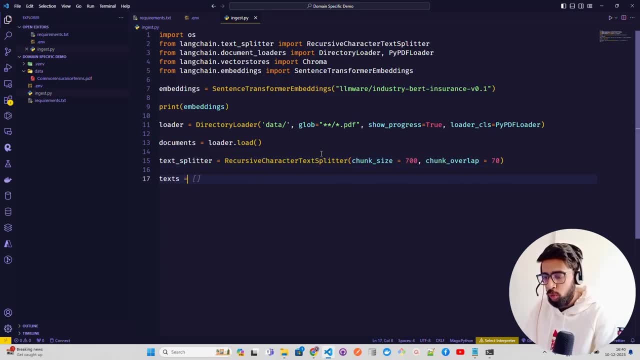 tenth of the chunk size now once that is done let's do a text equal text splitter dot split documents it's a method documents and this will and let's pass your documents 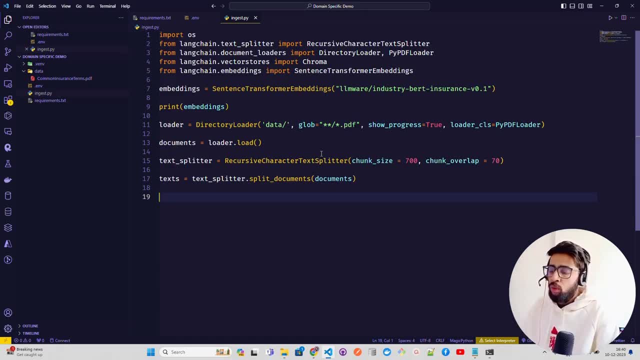 this is fine now we are done with that after that let's do a print thingy here print text something like this i don't know we'll 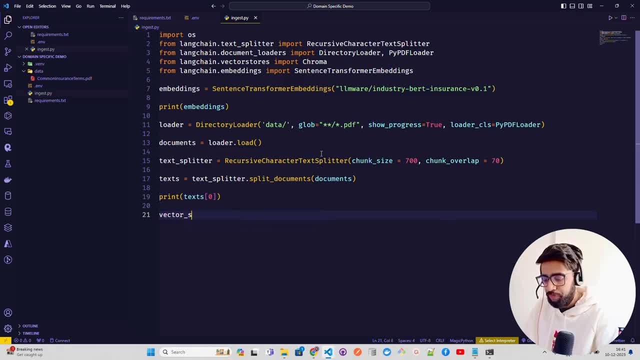 check it out okay now the next is let's have a vector store or vector stores and here i'm going to use chroma but you can use any other as well chroma dot from documents from documents to do and then you pass your text you pass your embeddings thingy and i'm also going 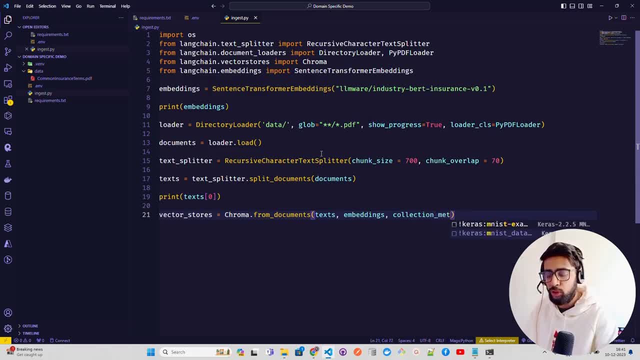 to define a collection metadata or i'm creating the supports you know ip dot levinstein cosine blah blah blah right so you can look at i have explained that in my previous videos a lot i'll recommend you to watch that if you have some time hnhw and then hnhw 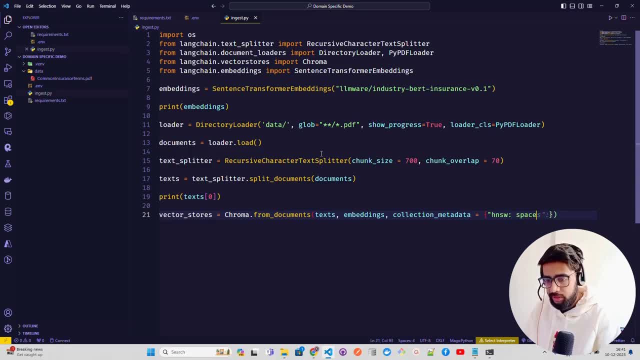 it would be in the same one hnhw and then space now i'm saying okay you use hnhw hnhw sqlflow hnhw sqlflow sqlflow sqlflow 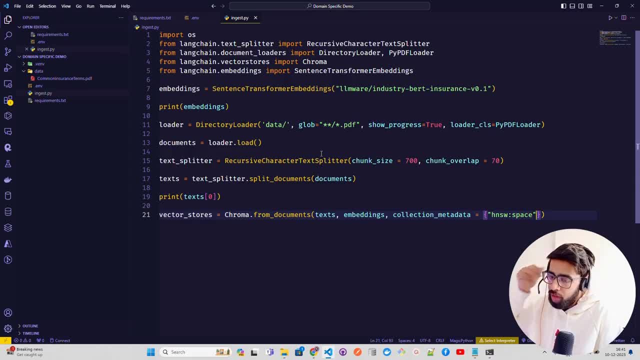 And then it would be nothing but your cosine. I want to use cosine similarity here. Okay, now cosine. 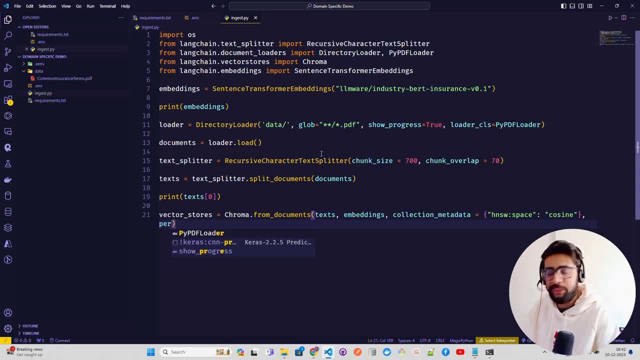 And then after you do cosine, let me do an alt G. I also want to persist this on my memory. So on disk. 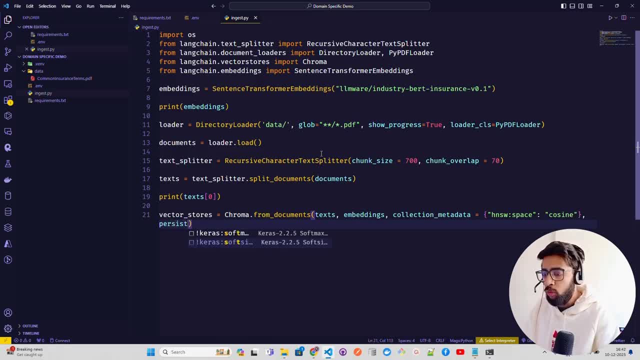 So let's do persist directory. Because I don't want to create embeddings on runtime, right? I want to persist that. 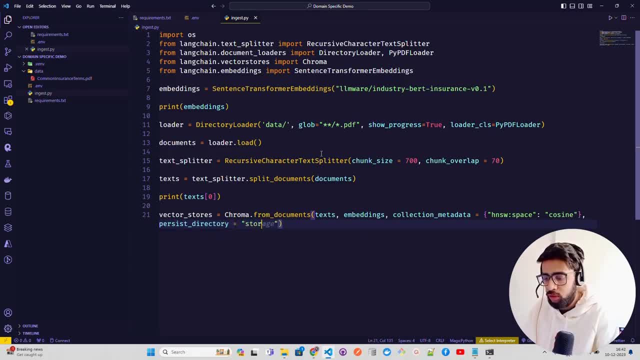 Okay, so persist directory equals. Then you have your stores. 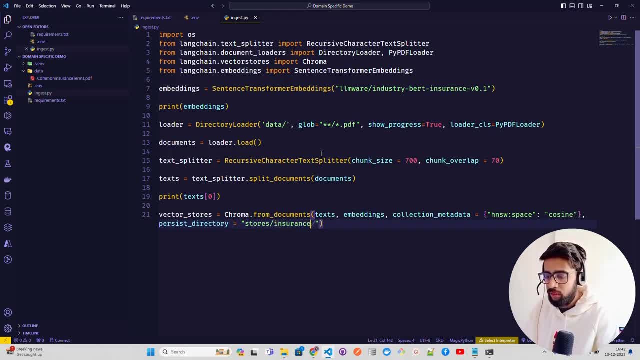 And then you have your, let's call it a name, right? Let's create a folder and it will create something here. Okay, so cosine, blah, blah, blah. 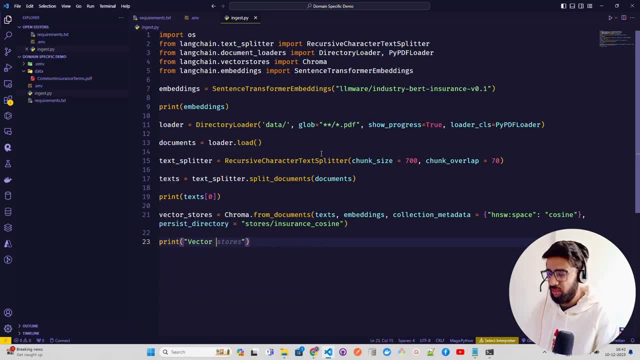 And just let's do a print and say vector stores created. 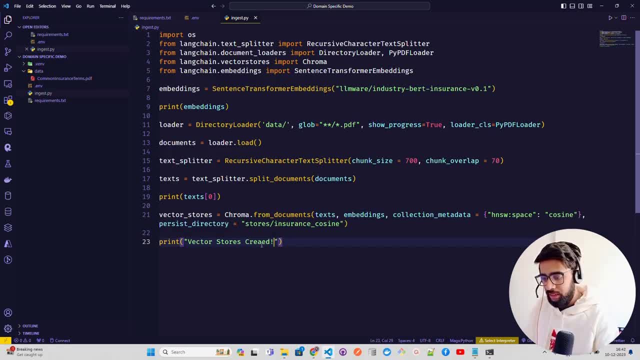 Okay, let me explain that quickly what we are doing here, guys. You know, if you are not familiar with the retrieval part of it. We have imported all the required libraries. 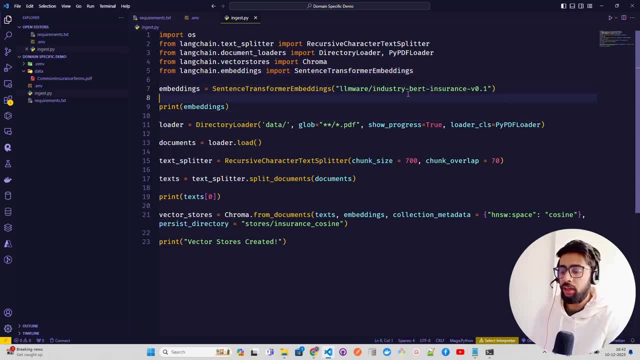 We have an embedding model that we are using. It's by LLMware by AI blocks. Okay. So I like them. What are they doing, right? 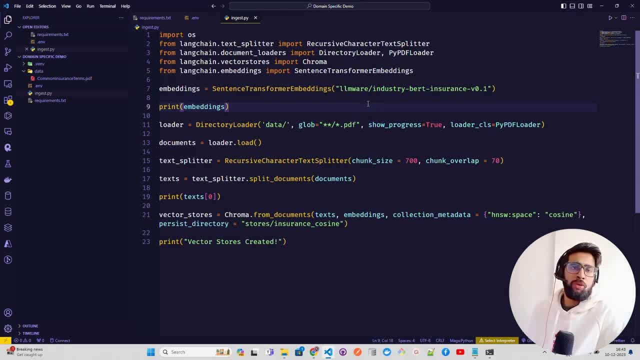 Basically, I like people who are working for the open source community to strengthen the open source, right? Because open source will win. That's how the AI, we have seen how AI has evolved, right? We still use BERT. 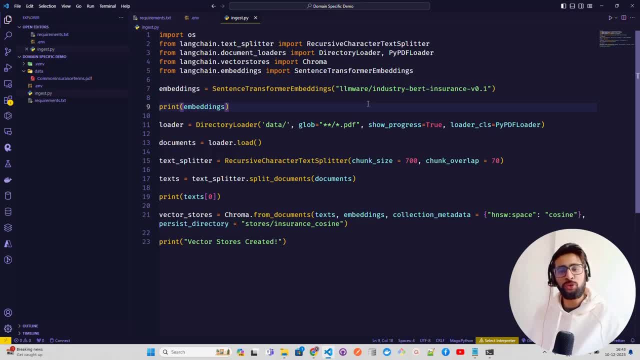 We still use Transformers. All these LLMs, even the closed source ones are based on Transformers, which is an open source thing, right? So open source is powerful and we have to make it even more powerful. 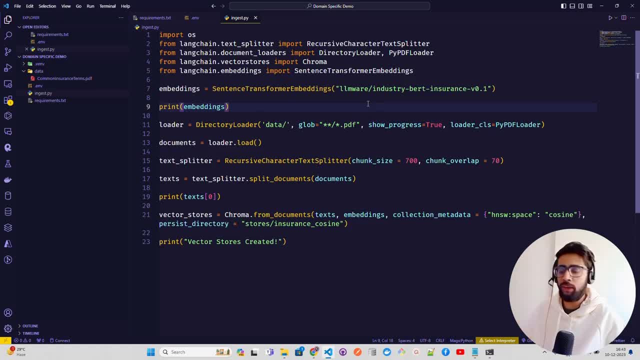 That's what the people like Jan Likun and others, they advocate it for, right? So LLMware, you know, the AI blocks or something, if I remember it exactly, they are doing good stuff. Let's back them up so they can build it more LLMs and more embeddings more and more AI products for us. 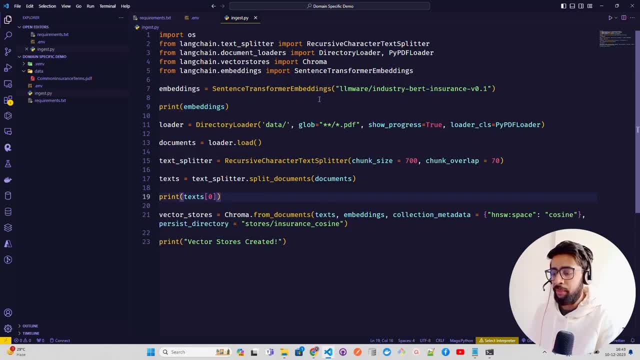 Now, if I look at here, we have an embedding model. We have a directory loader that loads your file and the documents loading it. Recursive character text splitter, you know, LinkedIn provides character text splitter, recursive character text splitter, JSON splitter, tick token. Uh. Etcetera. Right. So you can use that depending on your use case. 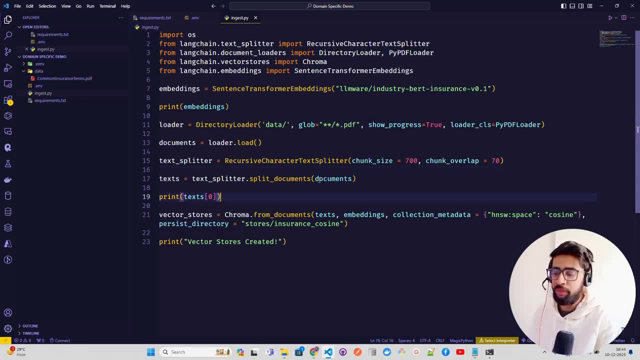 I have a chunk size of 700 overlap of 70. Then I'm splitting the documents. 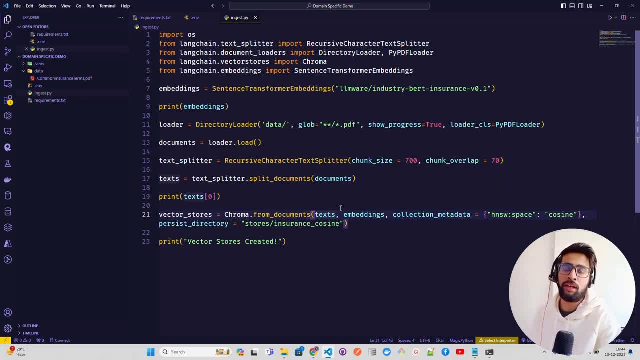 Then I am just creating a vector store, a persisting gate with a collection metadata. That's what I'm doing. 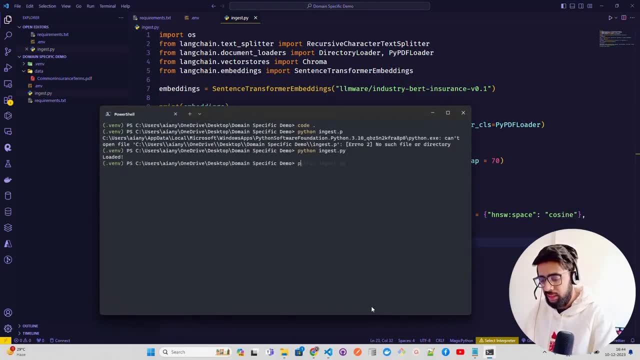 Now let's run this and see Python. Okay. Why I'm writing it. 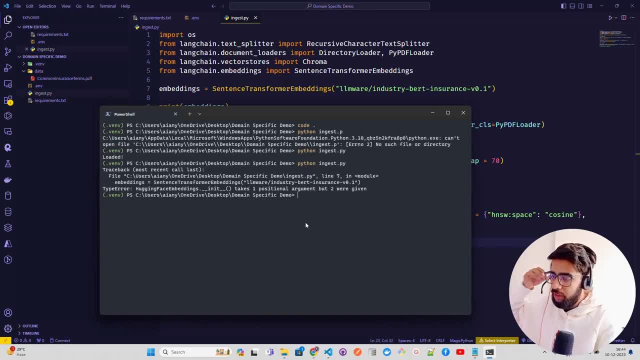 It says, uh, okay. Uh, LLMware sentence position argument two were given. Okay. I forgot to define the model name here, by the way. Excuse me. Sorry. 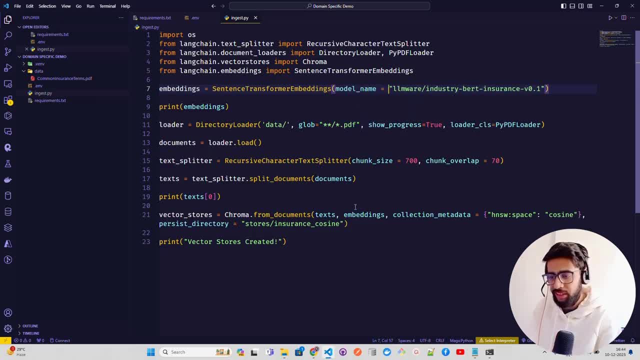 Uh, model name equal, but this is so bad, you know, it's automatically when there's a string, it should be model name. 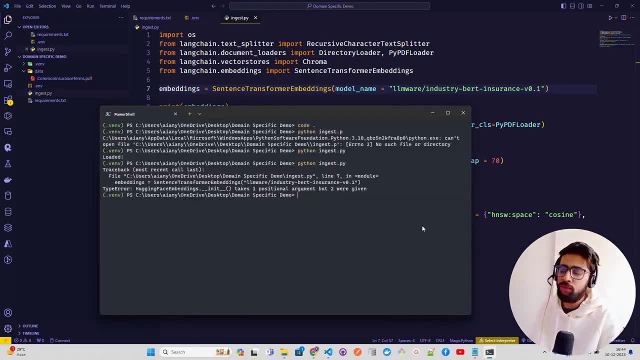 Right. But I think there's, there are other arguments and quarks as well. That's why I think the error is fine. I think that's, that makes sense. 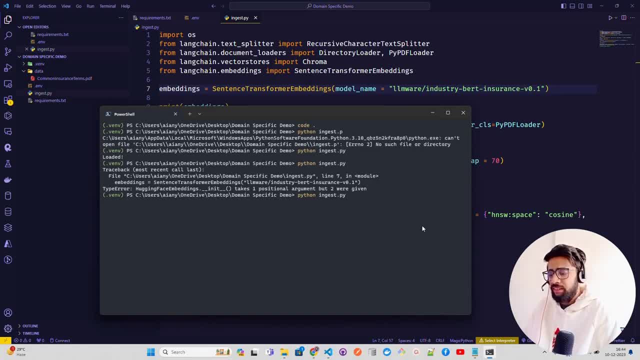 Uh, now once you do that, you will see, right. 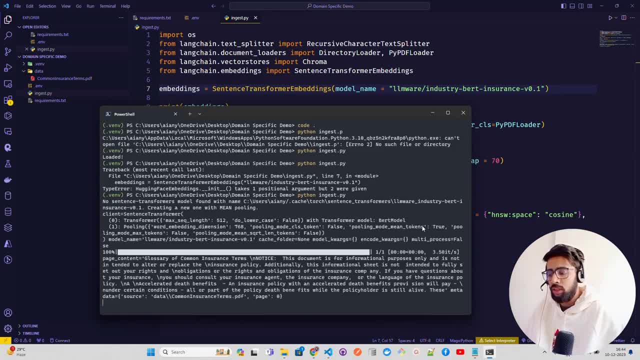 For the first time, it will take a bit of time because it's going to download the model for you from the hugging face weights thing. You can see it downloaded for me, transformer, pulling, et cetera, that they are using. Right. 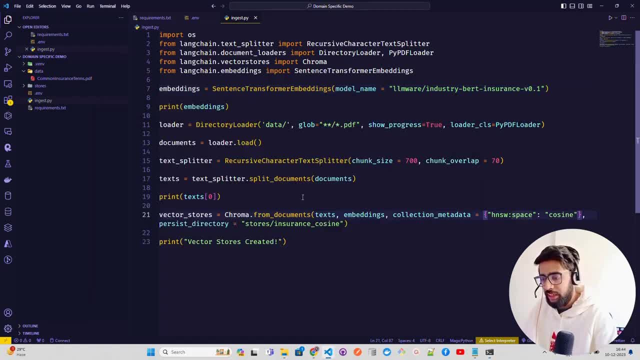 And, uh, now once you do that, it says vector stores created. So our vector store has been. It has been created and you can see it over here. 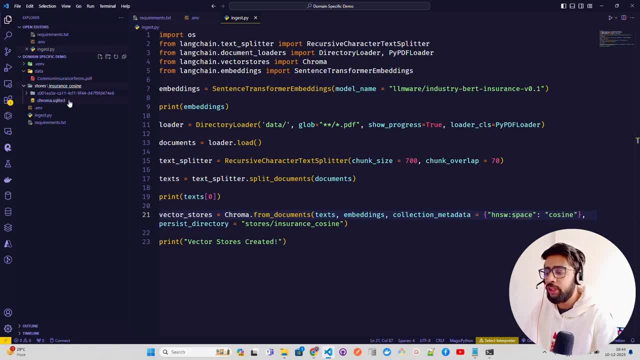 It says insurance cosine, you know, it has an SQLite database, uh, six months back. Chroma was using duck DB, park it right. Duck DB. They were using it. Then they migrated from duck DB to SQLite. And that's why you see this new structure of chroma DB. And then you have your everything here. 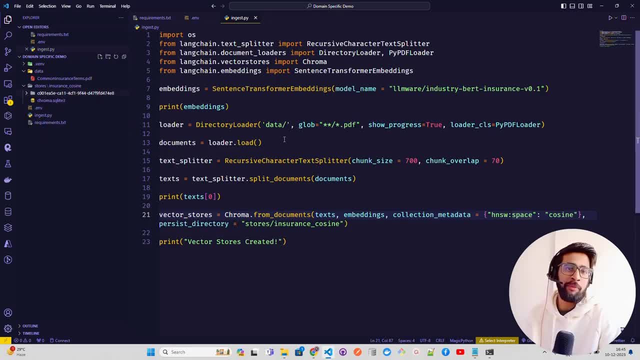 Okay. Your bin files, all the end dimensional spaces where your vectors are stored, right. Uh, with metadata arguments, et cetera. 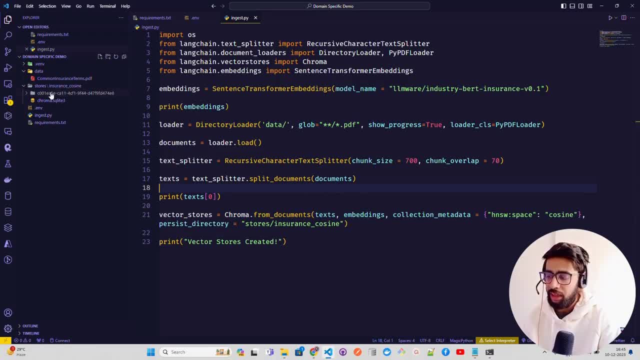 Now your vector store has been created, uh, which is inside this folder and our ingest is done. 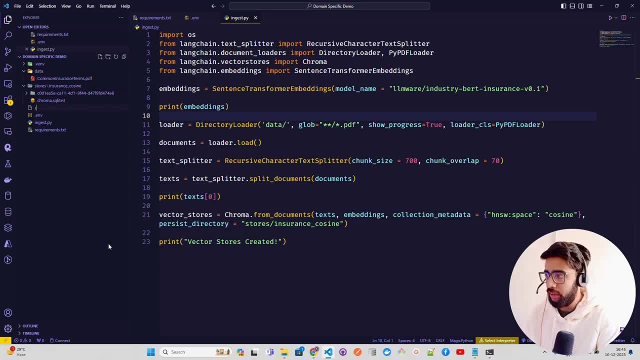 Now, once ingest is done, let's create something called retrieve now. 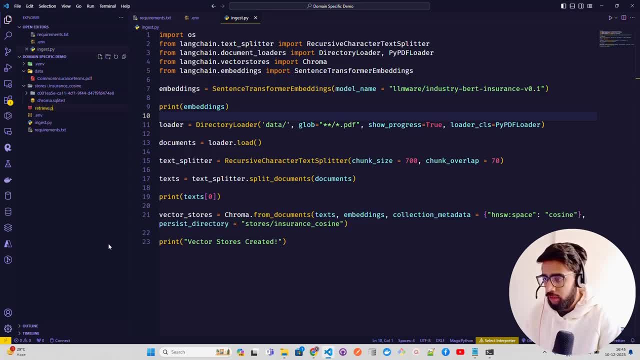 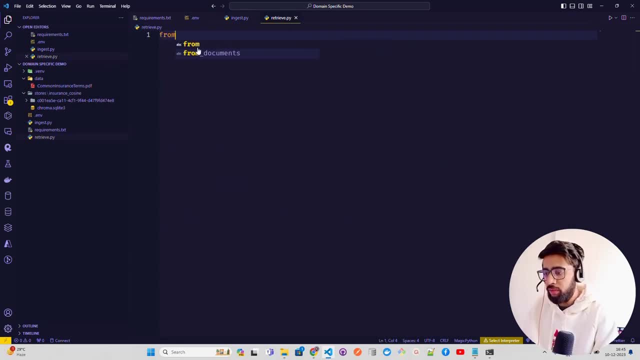 So retrieve retrieve dot PI or something. Okay. I'm just going to call this retrieved by now in retrieved by what we are going to do is we want to retrieve and see if our retriever is working fine. So let me just copy this quickly. 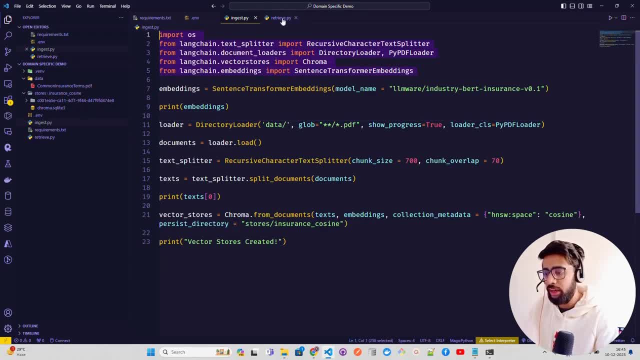 This thing here from ingest and we'll see what are the things required. Let me just put it here. 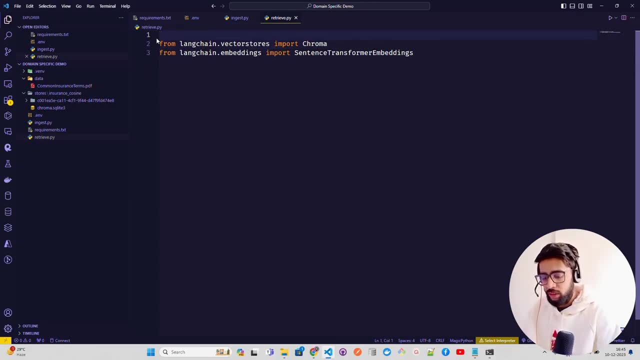 I don't need this couple of things, all of these, okay. I don't need it. Okay. 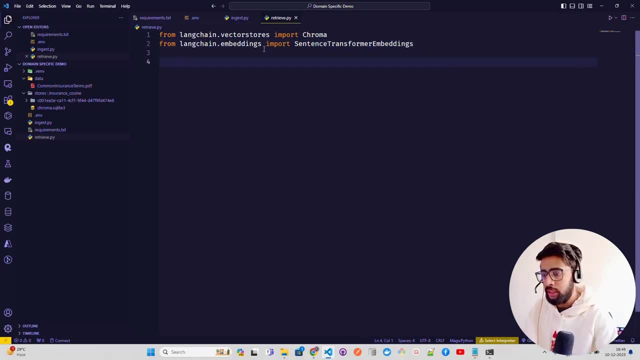 I need these two because these are the things that we're going to use. 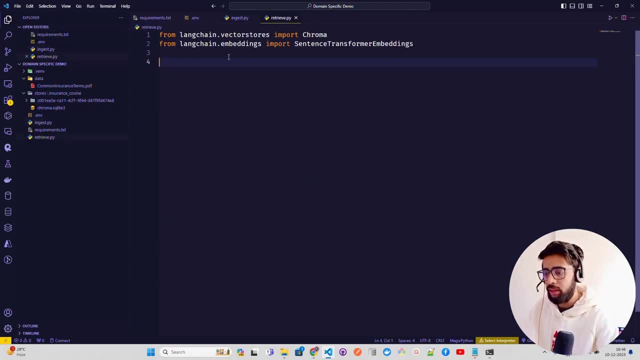 So I need the embedding model again, because once I put a query that respective embeddings needs to be there, and then we will pass that, uh, respective embedding for the query in the vector database or a vector store. And then that will retrieve the similar chunks for you. That's what we're going to do. 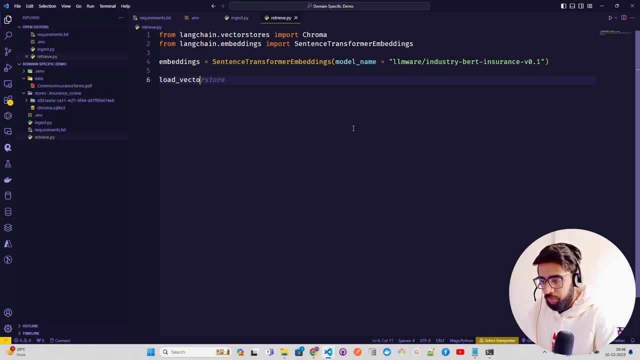 Uh, let me just do a load vector store here, a load vector store. And here I'm going to write chroma and I'm not doing from documents. You only do from documents when you are creating it. Once you persist on this, you just have to use chroma, not dot from documents. That's not required. 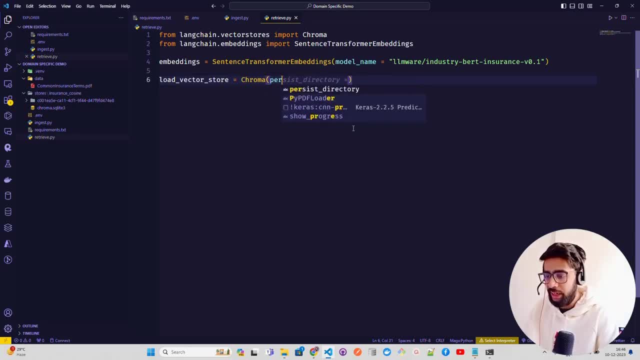 Now inside chroma, what I'm going to do is persist directory that which directory I'm going to use as a vector store is stores and in so rents cosine. Okay. You can look at the folder name there. Let me see that instance. Go. And then we have. 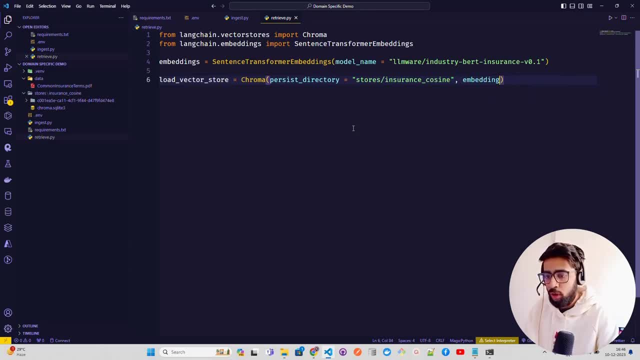 We have your embedding function, which is your model by the way. 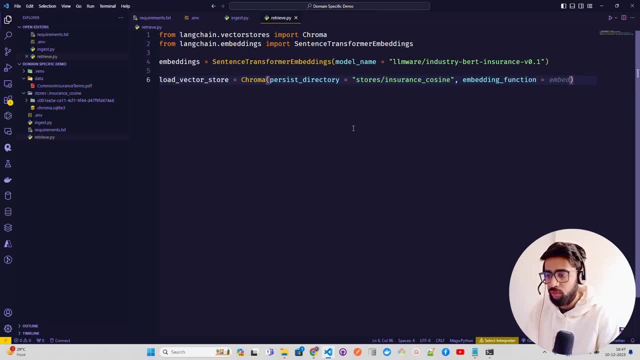 So that's called function here in this class of chroma, and then you pass your embedding thingy. So let me just pass that. Let me do an alt G. This is how now you have loaded your vector store. 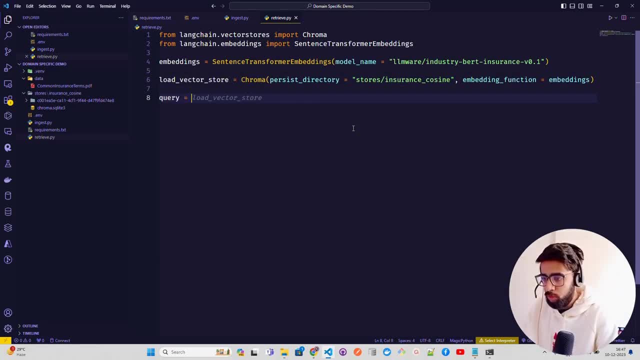 So once you load your vector store, let's define a query. So I'm going to use the same query I have here on the notepad, by the way, that I was showing you, let's just get it and you can use any other questions from your data. 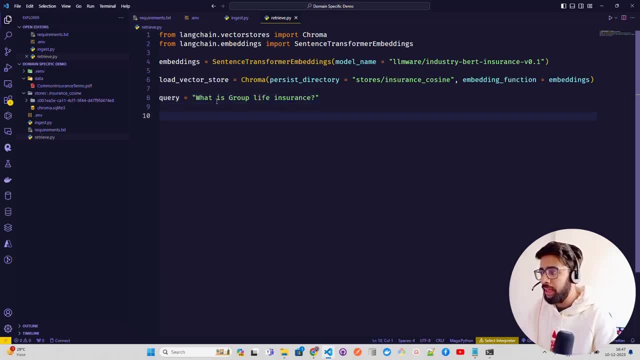 It's fine. Just to save some time. I have just already copied it. 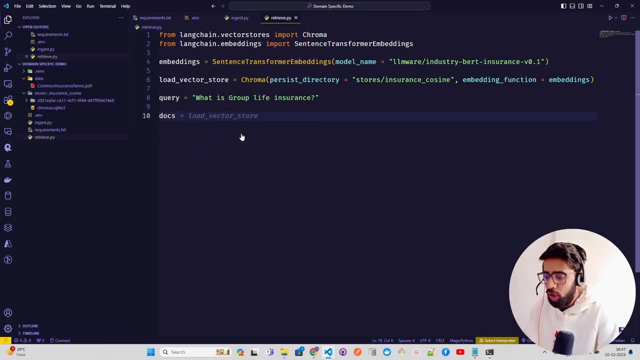 Now, what I'm going to do is I'm just saying docs equals load vector store, and it has of method that's called a similarity with a similarity search with the score. So I'm just going to do a similarity search to see if that is working fine similarity search with the score. 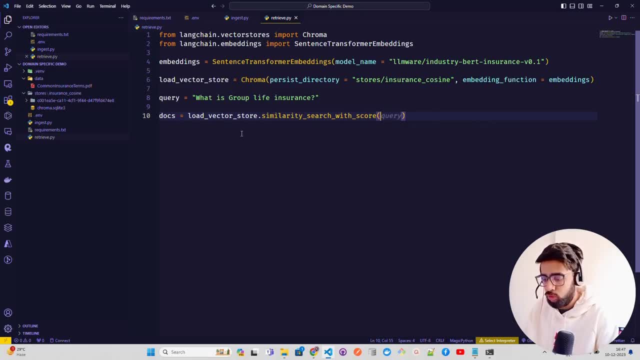 And that will basically return me the similarity search with a score. 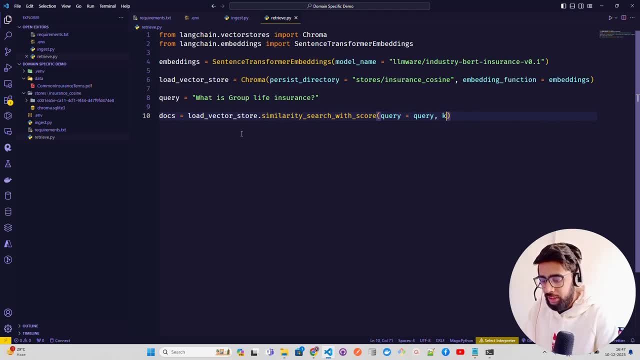 I'm going to define query equals query, which is, and then top K documents equal to. So give me three documents, and then I'm going to use a for loop for I in docs, just to make it more readable doc and score equals I Python is fun, right? I, and then print and, you know, some key value pairs here. 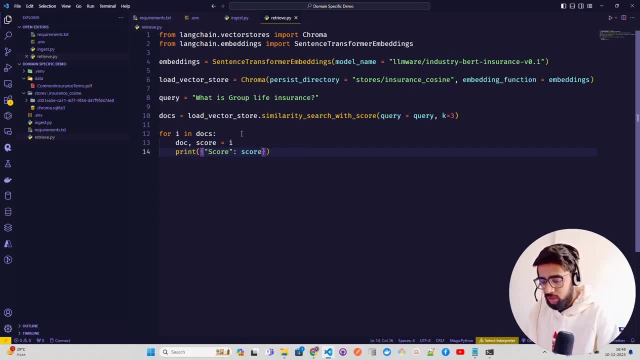 So let me just do a score and a score is done then content. So content equal, which is nothing but your doc dot page content doc dot page. Content, and then your metadata. So let me just do a metadata thingy here. So may it, uh, data, okay. Doc dot not paid metadata. It's only metadata. Okay. So let's just do that. Perfect. Let's see if this works guys. 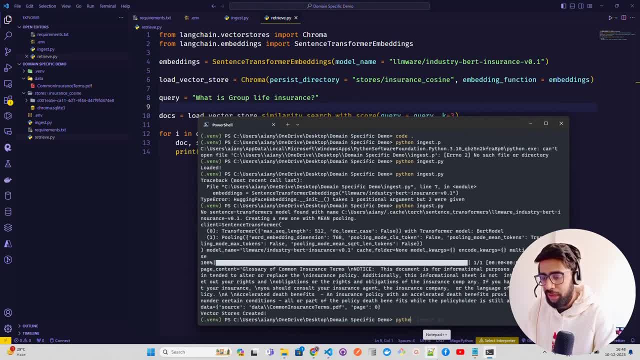 If it doesn't work, then see that we, I'm doing something wrong. So let me just do Python retriever, not re uh, excuse me. Ah, and it's not retrieved. Okay. It's retrieval. Let me see if the spelling is right. T R I E V E. 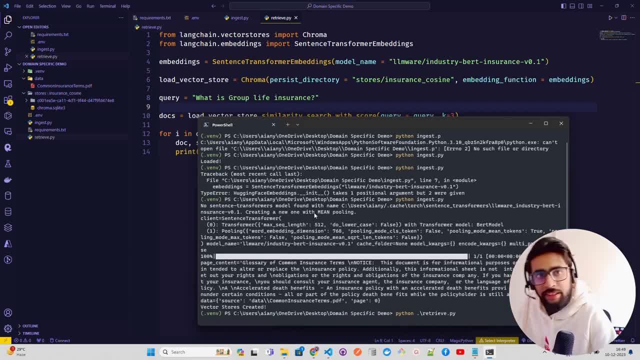 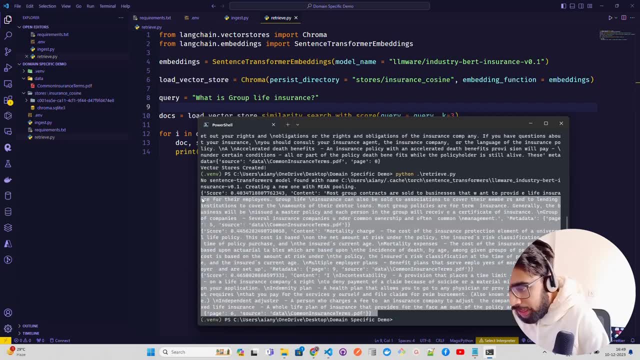 Once I do that, hopefully I'll get something here. Let's see it. Uh, I'm expecting that it will generate some response and you can see, let me just bring it here in the notepad. Okay. Uh, so you can read it better. I'll make it bigger. 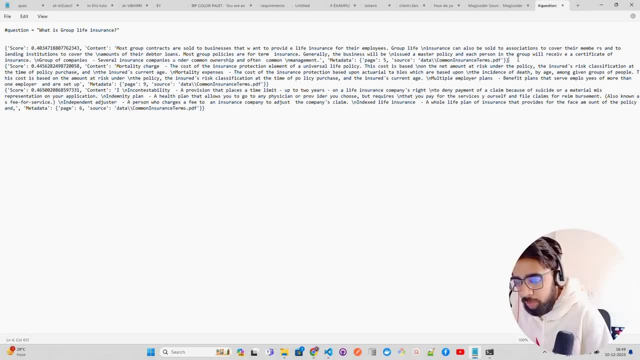 And. You can see here, let me just make it a bit space because we have top three documents and you can find out, we got our response. 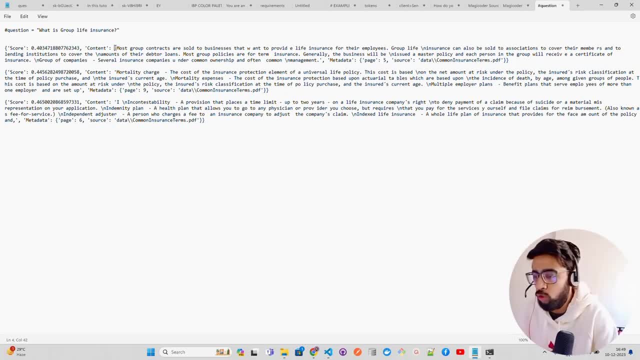 Fantastic. It says most group contracts are sold to business that are on a provide life insurance, blah, blah, blah. Group life insurance can be sold to associations to cover their members and lending institutions to cover the amounts of their debtor loans. And this is exactly what we see here in our data. 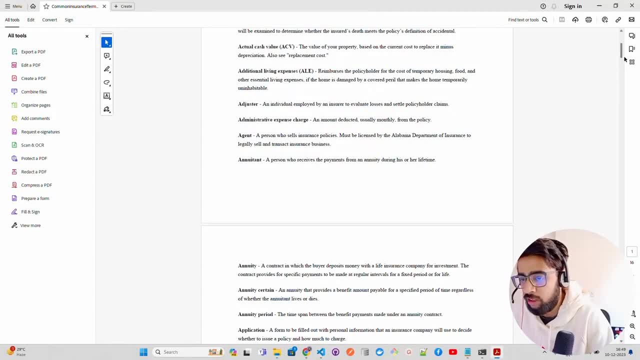 Let me open that and let me show you it's by group, right? Let's come to G quickly. Okay. Now G or something, and you can see, this is what it is. Group life insurance. 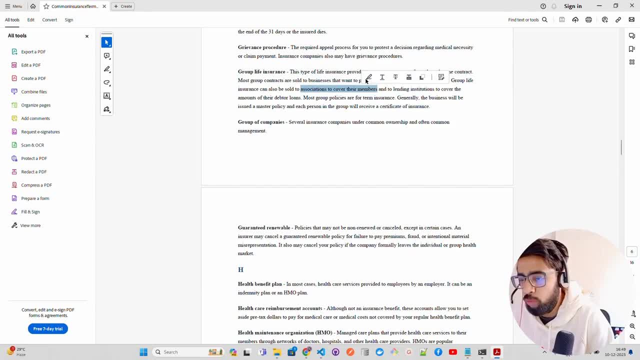 It says, blah, blah, blah, you know, most group contacts are sold to businesses that want to provide, you know, life insurance. You can see members, et cetera, right? Fantastic. 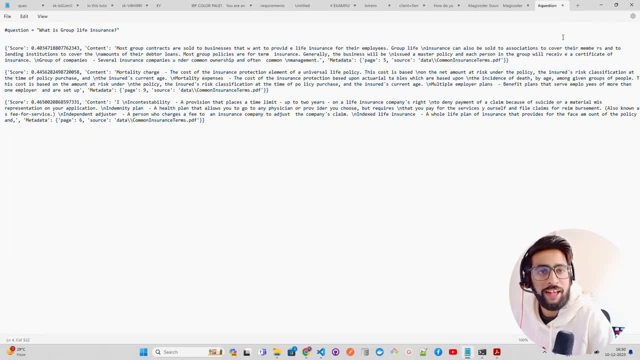 Well, it's working fine. Now the embedding model has done its job and you can see with a very small embedding model, it's done the job for insurance, understand the taxonomy and the terminologies of insurance industries. 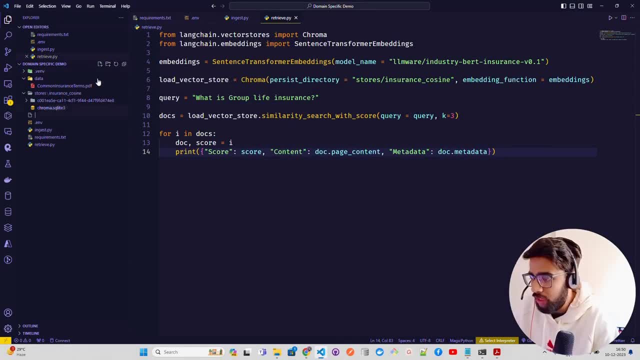 Let's go back and write the app dot PI thingy now. So let me just write. An app dot PI here quickly in app dot PI. What I'm going to do is I'm going to copy a lot of things. I don't want to write the same thing again and again. Okay. Now let me go back to my, any chat bot. 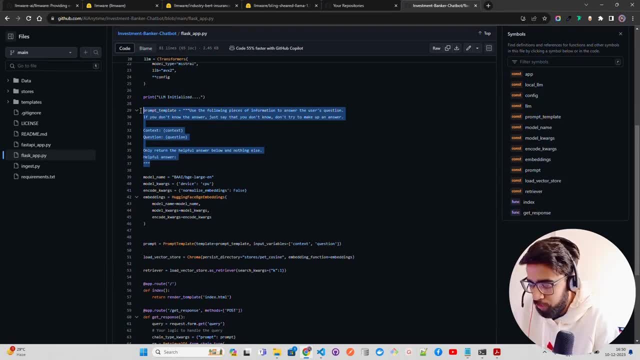 I'll just copy this prompt template, et cetera, right? I'll just copy this prompt template from my 25 others, drag a video that I have. 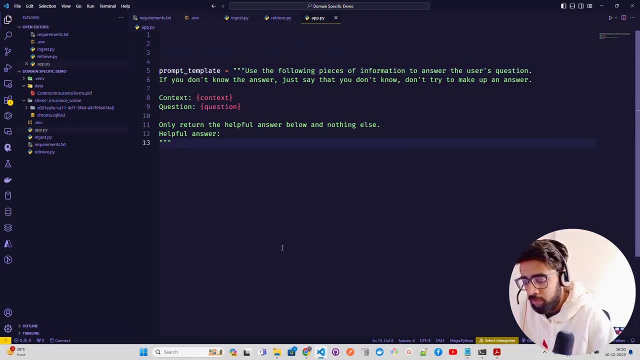 Okay. I'll just copy the prompt template, a simple prompt template, and a few things I will also copy. I'll copy this. Yeah. Let's copy this. Load vector store as well. Exactly. Let's copy this too. Okay. Uh, and you know what we are doing here. 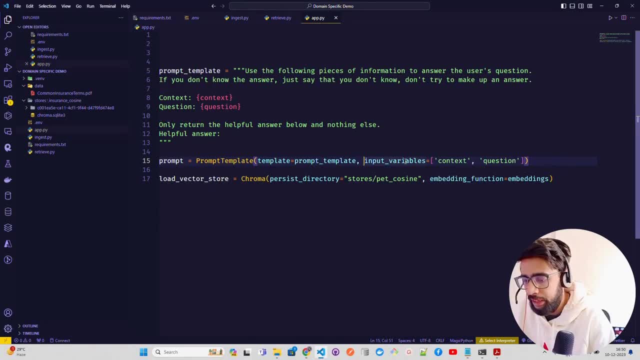 So we are just using a prompt prompt template template equals prompt template input variables, context, context, and question. Then I'm loading the vector store chroma. 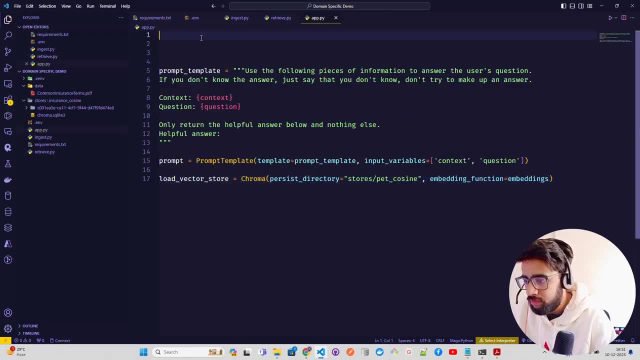 Let's get it from here quickly and put it here. 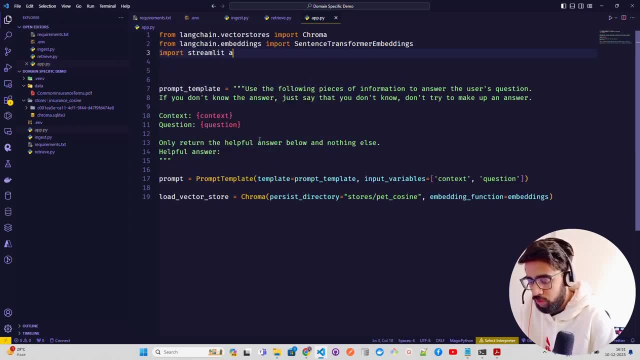 Then let me just import streamlit as well. So import streamlit as ST. 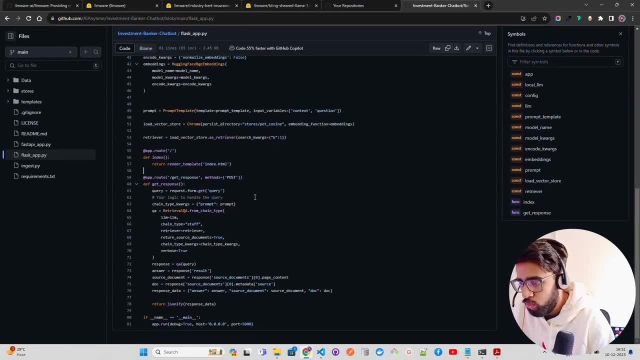 And then what I want to do is next. Let me just get this as well, and this, I will write in a function. 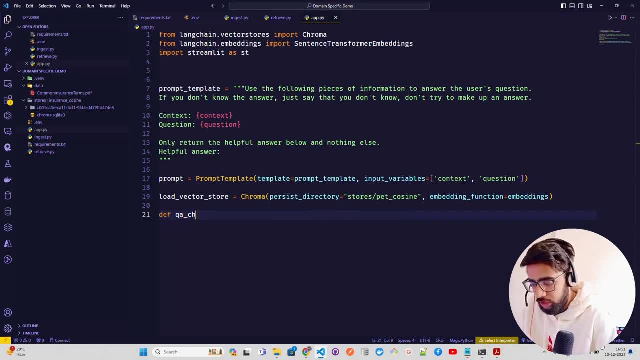 I'll explain that, uh, from top to bottom and bottom. Let me just write a QA chain and inside this QA chain. I'm just going to use that. There are some indentation problem. Let me just get it back once. 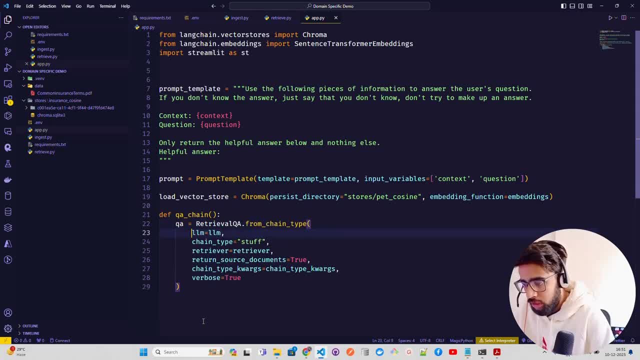 And then I can just do this as well. Once perfectly fine. And just, just return the QA. 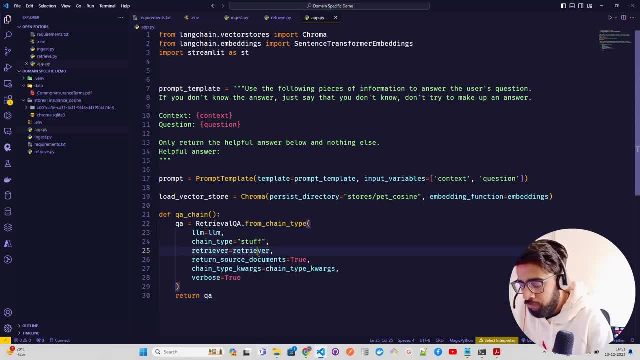 Now this is going to be the same guys. You can see we are, uh, Oh, okay. 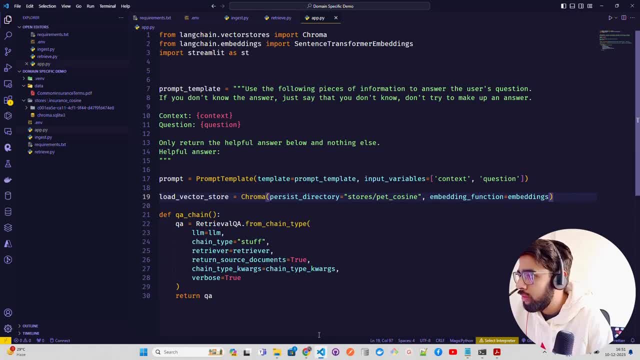 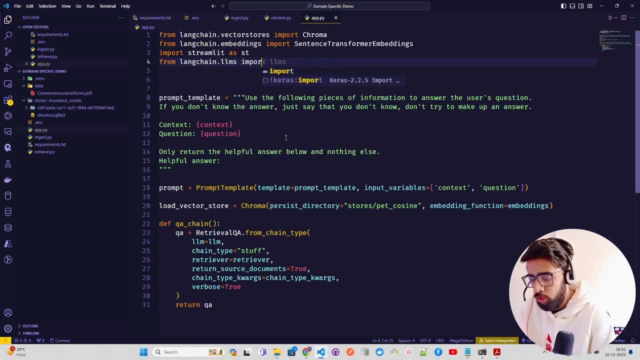 Uh, a lot of vector store and then let me just get a few things quickly from Langchain dot LLMs. Now here in the LLMs, I'm going to import hugging face hub, right? I'm going to use the hub. 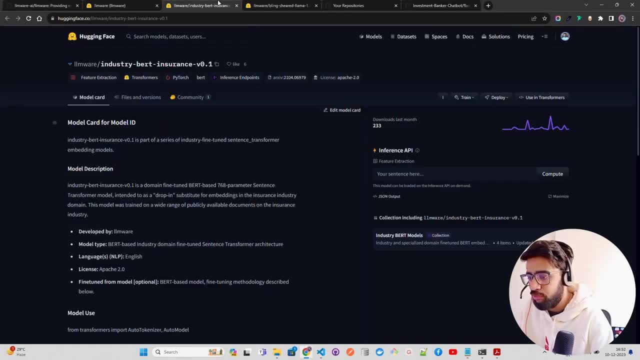 I'll show you how you can get that inference API. Now, if you look at this model, this is the LLM that we are going to use. 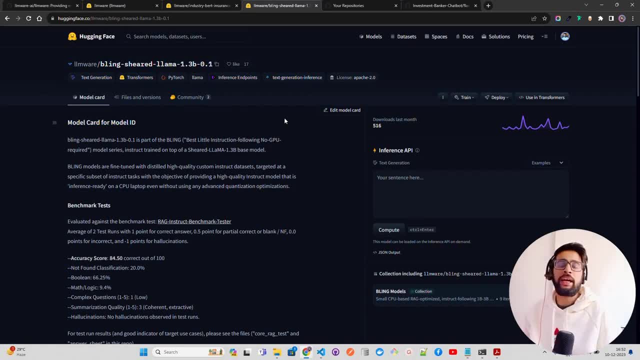 It's around 80% lesser in size. And it gives you the same performance as equivalent performance as seven B models. 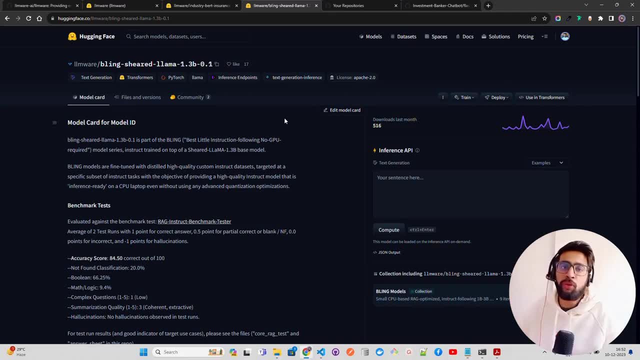 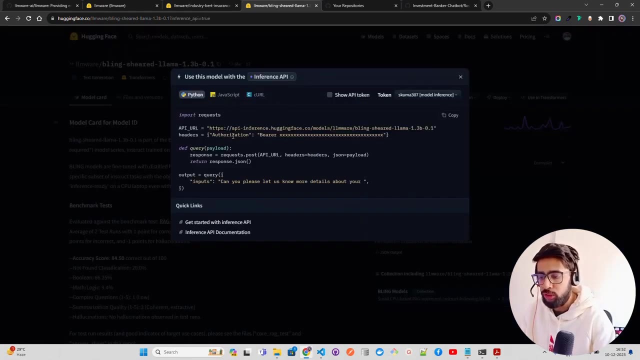 And that's why I'm using it because this LLMs are fine tuned for rag guys. So if you want to build a rag, you can just use this and you can see it's available through inference endpoint. You can find it out over here. It's also available through TZI text generation inference. And if you come here on deploy, once you click on this inference API, it also shows you that how you can use it through tokens. 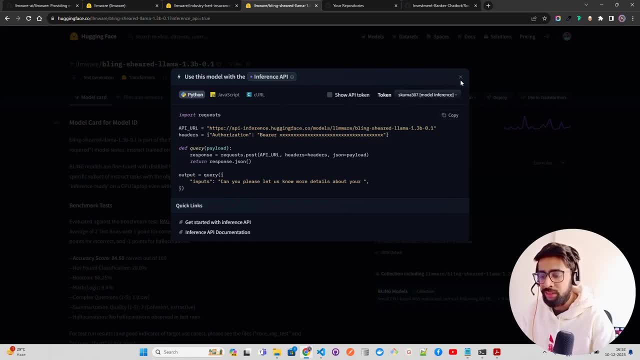 You know, so API tokens and blah, blah, blah, right? Uh, inference API. 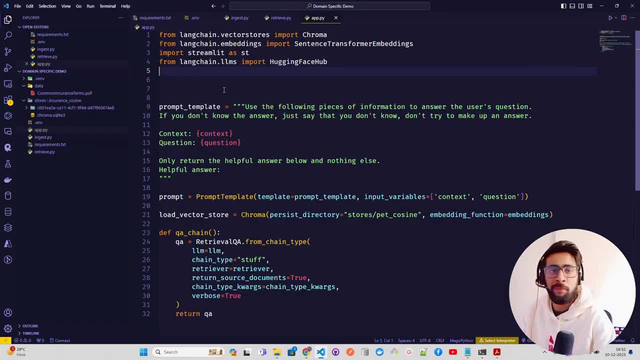 And that's what I'm using here. You need a token from hugging face settings. You go to your hugging face accounts, go to settings. If you don't have an excess token, create an excess token and just get it. Make sure that excess token is readable. Read, read only tokens. Oh, the right is not required for this purpose. 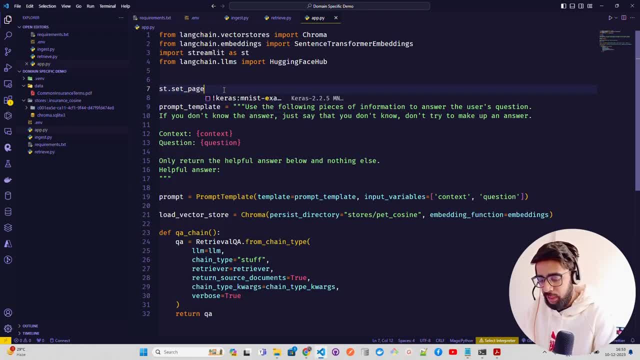 Now, let me do a set page, configure something quickly. Okay. Set page config for streamlit. 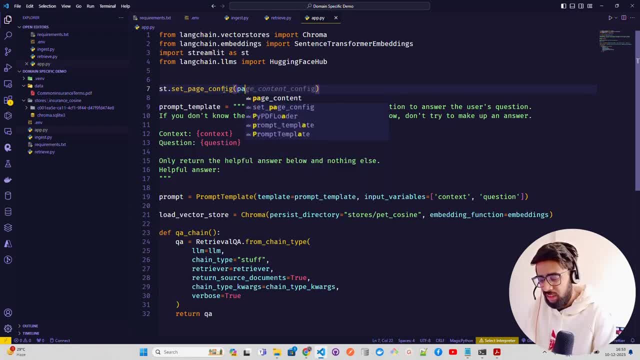 So ht dot set page config. I'm going to give a page title, uh, page title equals, uh, what would I do? Insurance. A rag demo. Okay. Uh, set page, config and ht dot title. Okay. 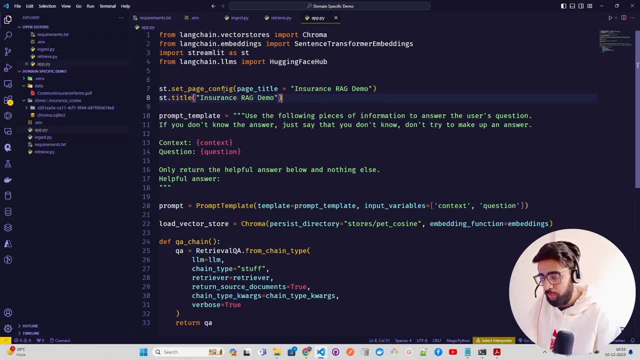 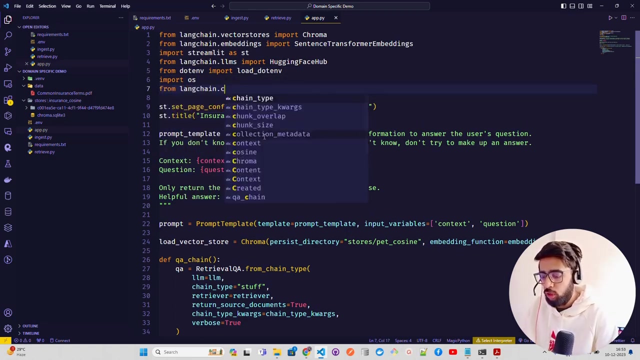 Uh, an insurance rag demo. Now I need a DOT ENV thingy as well. So let me just do, I have installed Python DOT ENV. So from DOT ENV import load DOT ENV, uh, load DOT ENV. Let's get OS as well, because we have to get ENV as well. Retrieval QA chain is required. So from langchain.chains import retrieval QA chain. What else we need? I think we are fine with this now. 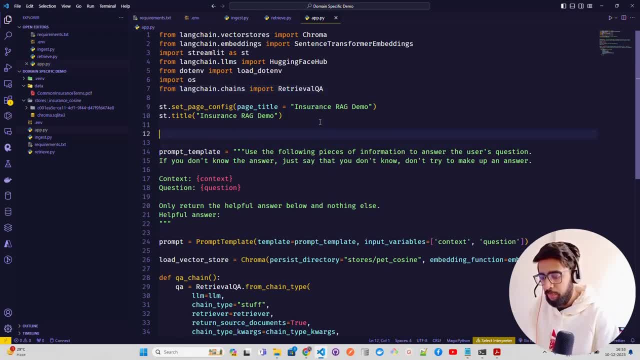 Okay. Uh, let me just get this load DOT ENV thingy here very quickly. Load DOT ENV. 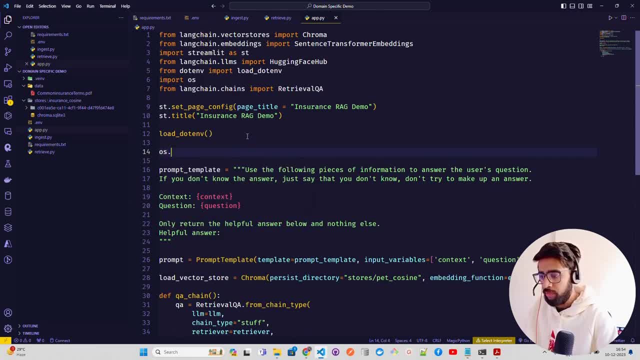 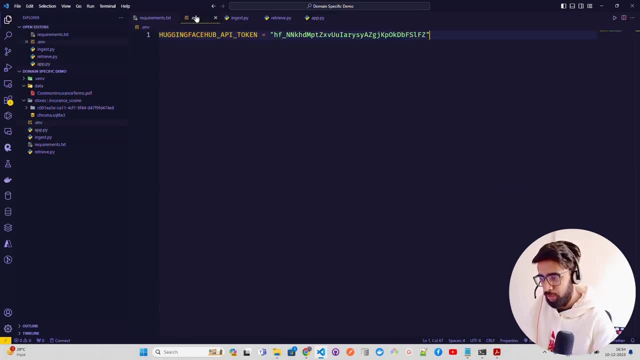 Load DOT ENV is fine. And then OS DOT envarn and here you have to write the same. Anyway, let me just get it because anyway, I'm going to delete that. Okay. So I'll just. Copy this variable. 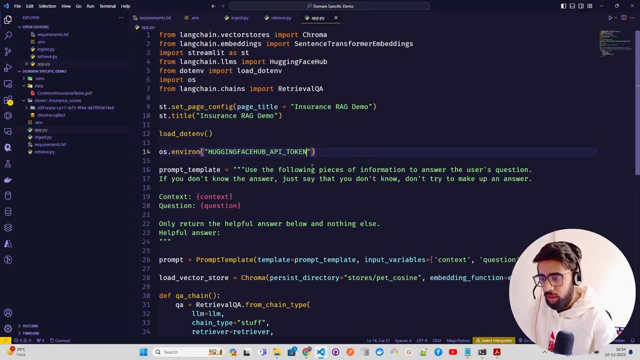 Come here in app DOT PI and then just paste this OS DOT get ENV perfectly fine. Now this, your API has been loaded. 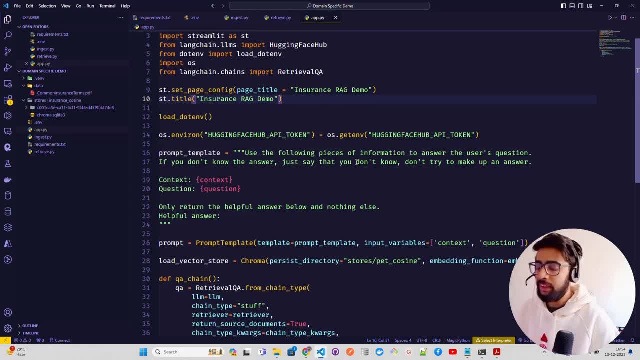 Now you have your prompt template set. Now, so you can basically increase the, uh, complexity in prompt templates to avoid hallucinations or make it more structured, or you can also specify some examples, uh, here just to retrieve better. Now you have your prompt you have. Let's get it from retrieve DOT PI. 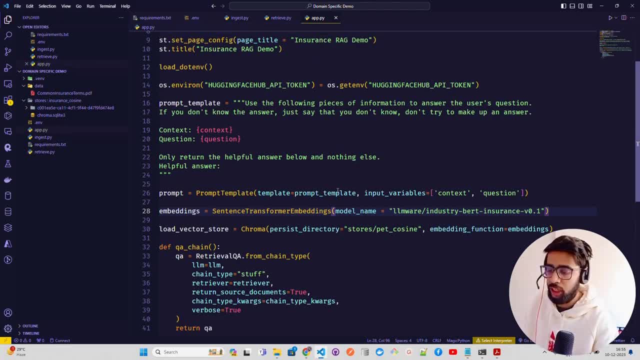 That's why I've written that function as well. Right now, it embedding sentence transform and embeddings model name is okay. 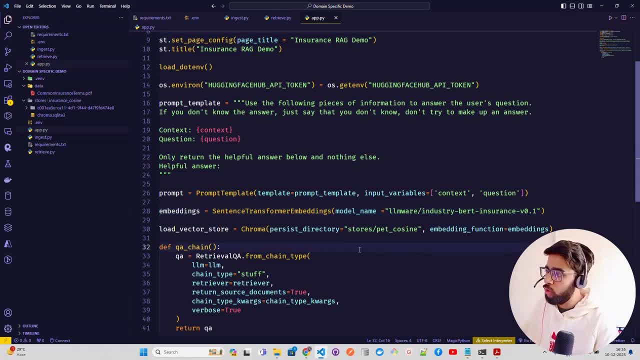 Uh, let me just look more better than load vector store chroma. This will not be paid cosine. This is from my previous repository. You have to change to your. Cosine. So. Insurance cosine embedding function embeddings, and then you write your retriever. 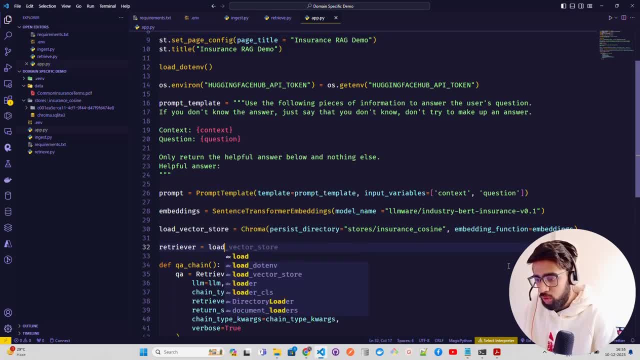 So retriever equals, uh, load vector store. Okay. 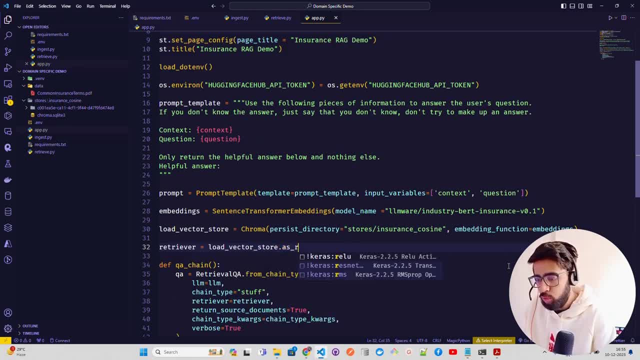 So load vector store and dot as a retriever. So I'm going to use as retriever, uh, offline chain. 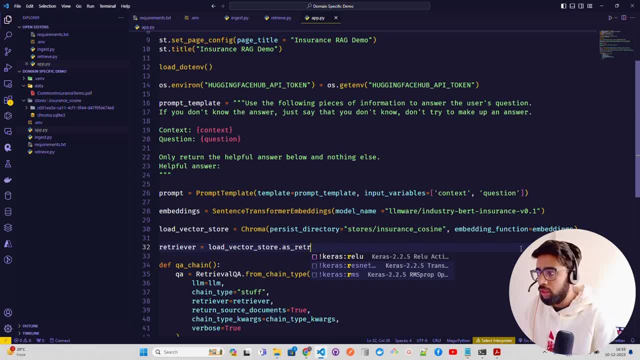 So as a retriever to, uh, I E V E R as retriever. And here I'm going to pass the search quark. 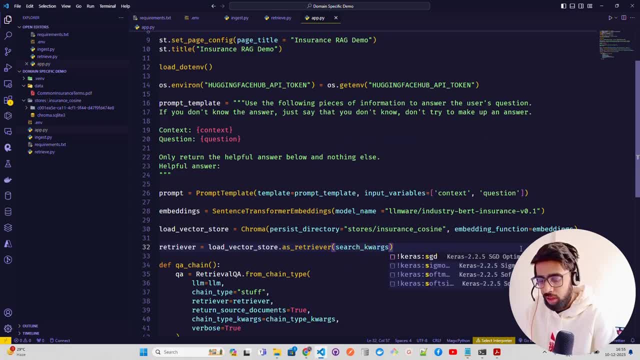 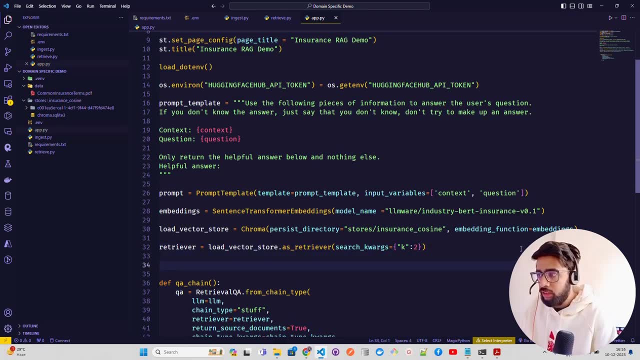 So search quarks means top K documents and some of the other. Uh, arguments that you can define now here, I'm going to go just do K equals to only look at two top K documents that retriever is done now here to define a repo ID for your model. So let me just do that for the LLM that we are going to use. 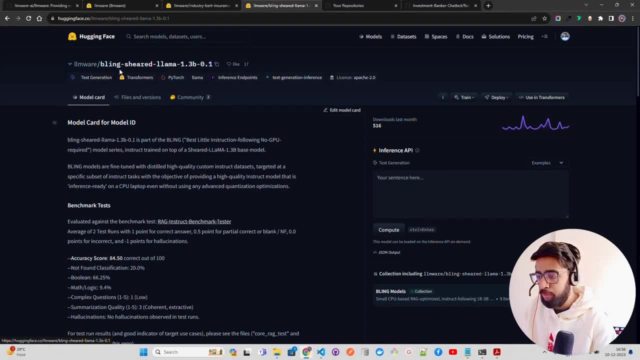 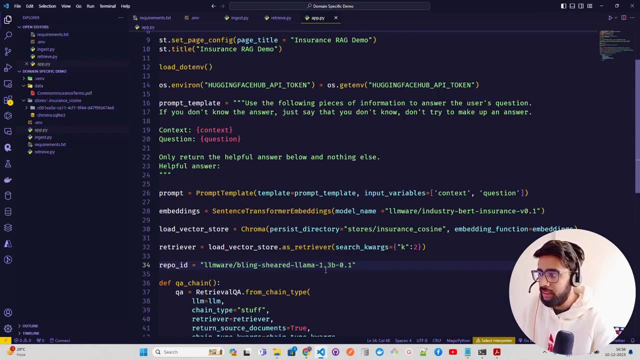 So this is the LLM by LLM, where you can see blinks here, the Lama 1.3 and the first version of the model 0.1 that you see now the repo ID is done now after repo ID, what do you have to do is you have to do LLM equals hugging face. Uh, so let's do an hugging face hub. 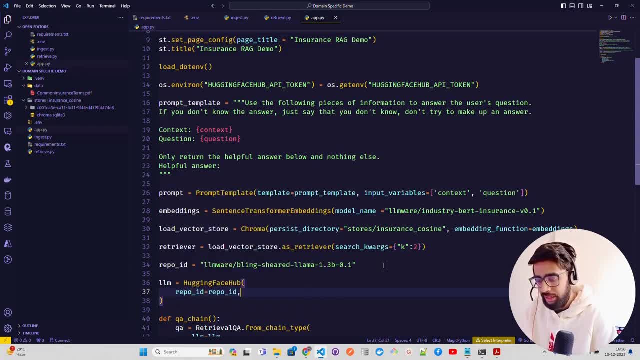 And inside this, I'm going to pass my repo ID equals to repo ID. Then you have your model quark. So let me just do model quarks where you can, you know, set up your inference parameters. It's not hyper-parameters either inference parameter that you can set up like temperature, top P top K max new tokens, et cetera. Okay. 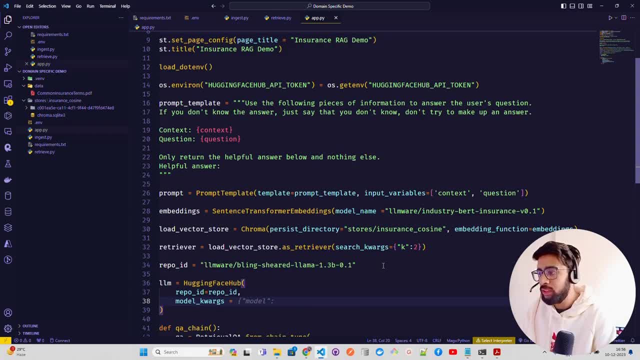 And these are the smaller thing that you should know guys, hyper-parameter you do it. Once you fine tune or train a model, not once you inference it now model quarks. And. 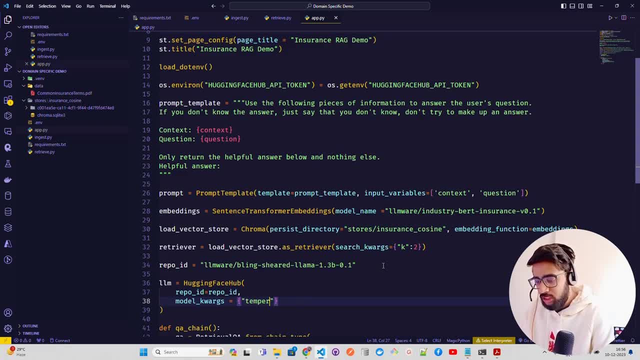 The model quarks, what I'm going to do is pass a temperature. So let's me just do a temperature and as let's keep it 0.3. Uh, it's the value can be, if you keep it higher, the model will be trying to become more creative, might hallucinate a bit, but it has, it's not strongly associated with hallucinations. I see a lot of people in industry talk about it, right? Uh, that you can, your temperature is higher model hallucinate. It's not like that. Uh, it has some role to play, but hallucination is a complex topic. Uh, max length 500, let's keep it, uh, a smaller max length. 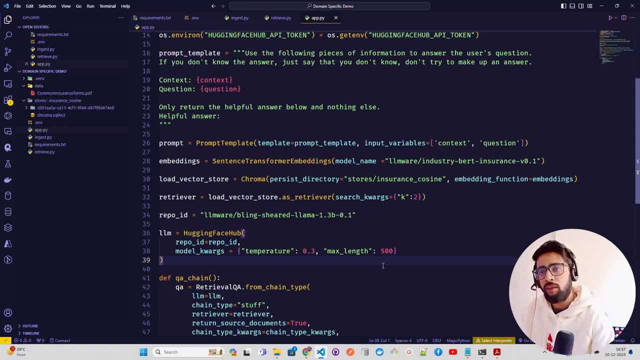 This model is good for chat, but kind of a thing where you want a very long detailed response. This model is not for you. This model is for, if you want to build a chat bot, uh, kind of a thing or conversational interface. 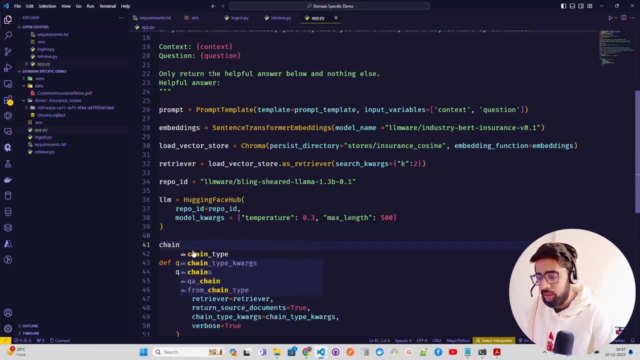 Now model quarks. Now, after that, let's define a chain type quarks and chain type quarks is nothing but your prompt thingy. So my prompt, okay. Prompt E. Well, a colon, by the way, that becomes your prompt that you have defined in line number 26. Perfect. 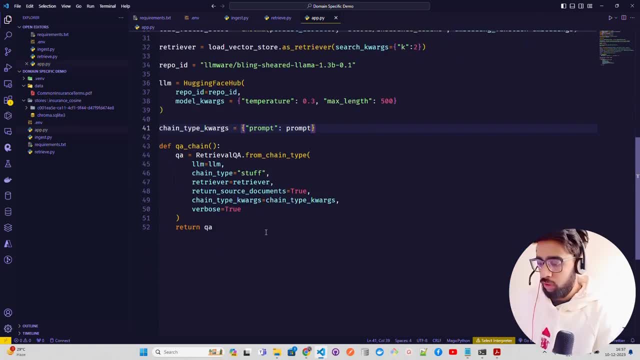 Then we have QA chain guys. And then after that, uh, once you have this QA chain, uh, let me just do a QA equals, uh, QA chain. 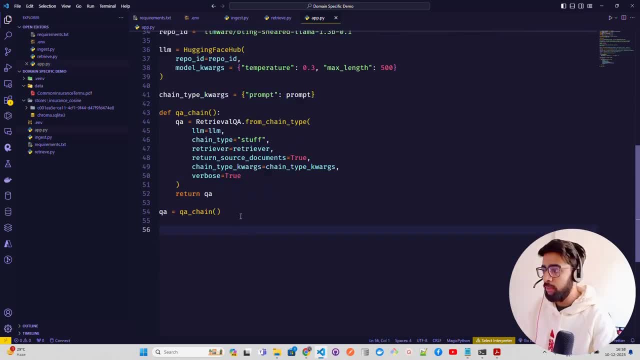 And then we are going to use this QA, uh, in our streamlit code. So let me just write a main function. So define the main. And let me also quickly write if. 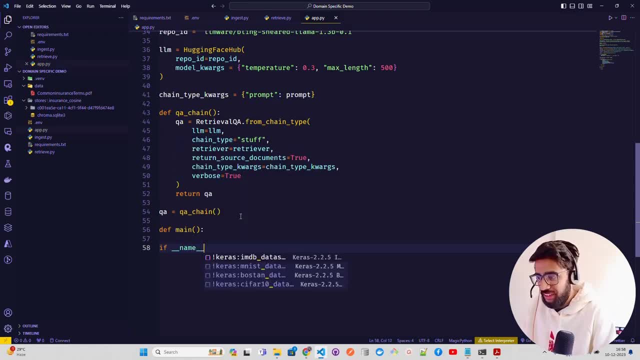 Underscore underscore name, underscore underscore equals. And this is bad, right? You can see it's tab nine is not suggesting me once I need it. 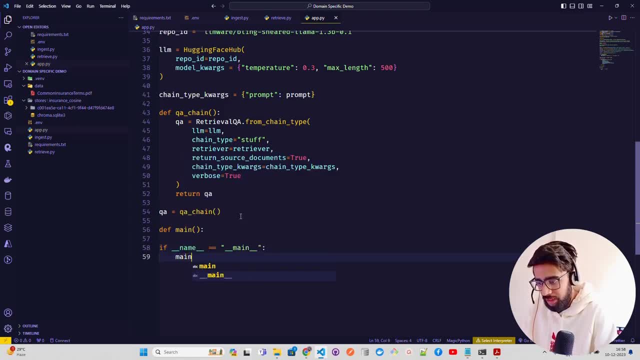 Okay. Main underscore, underscore, and then colon main. 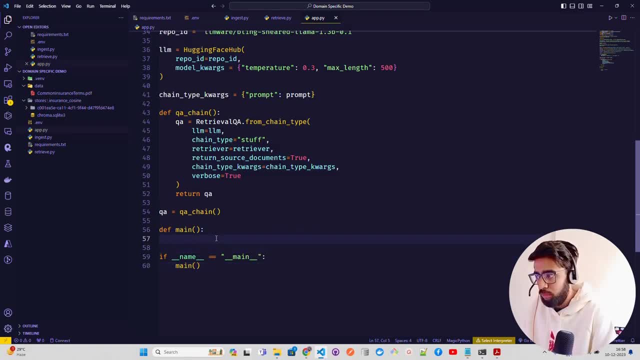 Here we go. Okay. Now inside this, I'm going to rise my, all of the thing. The first is text query, which is the text area. So HD dot text area. XT dot text area. And here I'm going to write. Ask. Your question. 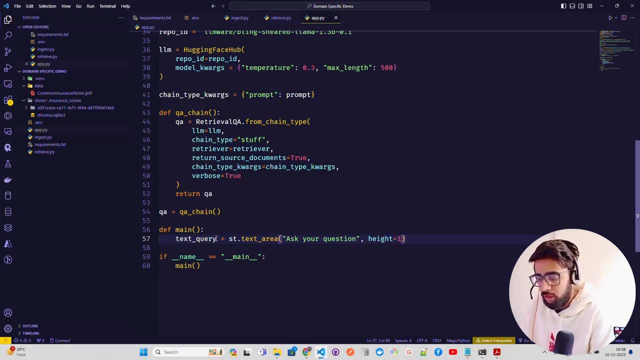 And let's give a height to it. So height equals let's keep it a hundred. Okay. It's fine. 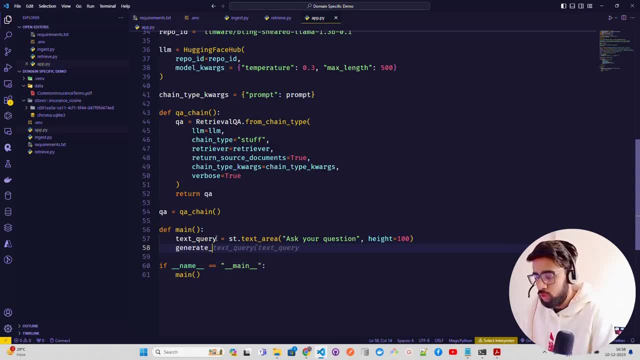 Hide equals a hundred. Then let's have a generate button response kind of a thing. So generate response button, generate response button, and let's define HD dot button. 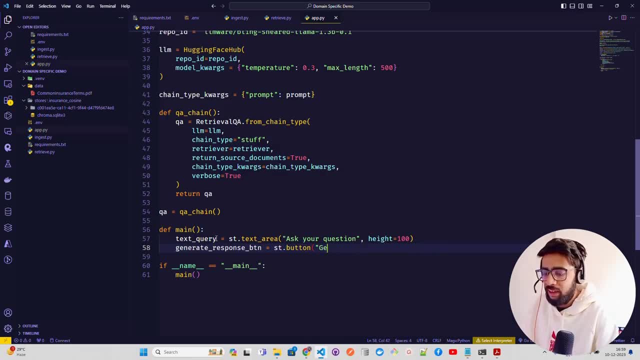 Uh, HD dot button generate response, or let's call it a run rag. Run. 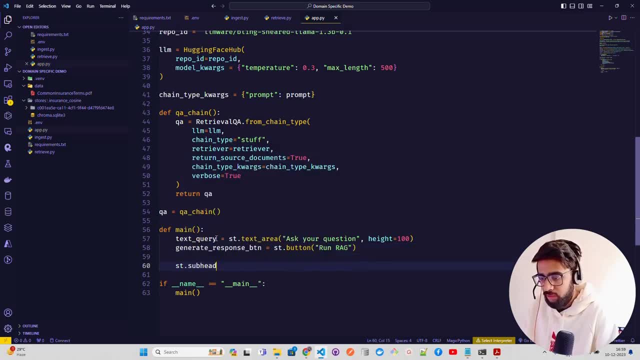 Now I'm going to say HD dot subheader, let's already keep a subheader for response and let's call it a response response. 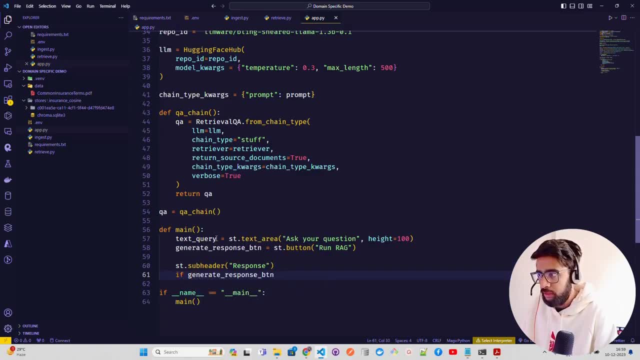 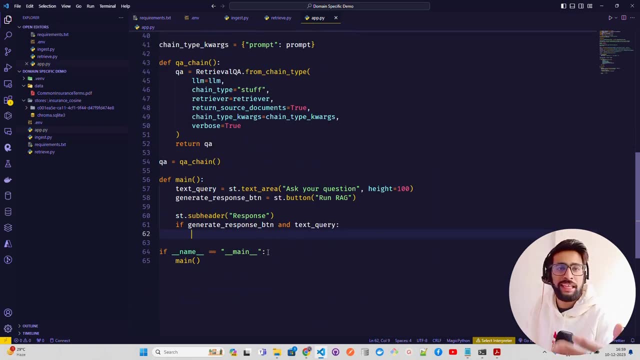 And then after that, I'm going to say if generate response button and text query, there are value or the button has been clicked. And there's a value inside text, but you can also do with length text query, greater than zero, or if text query is not none, you can also do that. 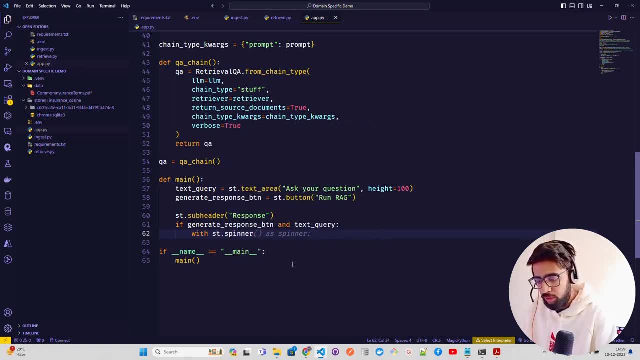 I'm going to have a spinner that will spin with. HD dot spinner generating response, a generating response, blah, blah, blah, with HD or spinner. 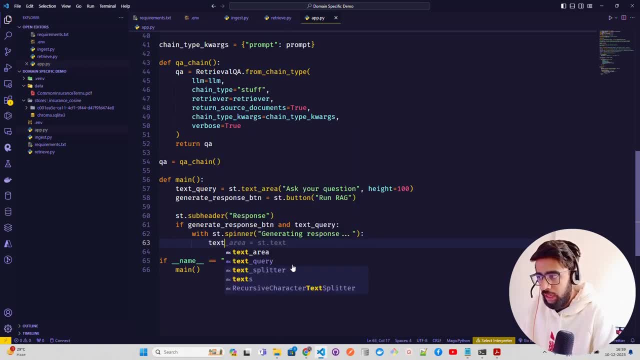 And then you just do, ah, with a week, then you write text response, text response equal. Then I'm going to use the QA that we have, you know, used above and pass the text query. Here we go. Text query. 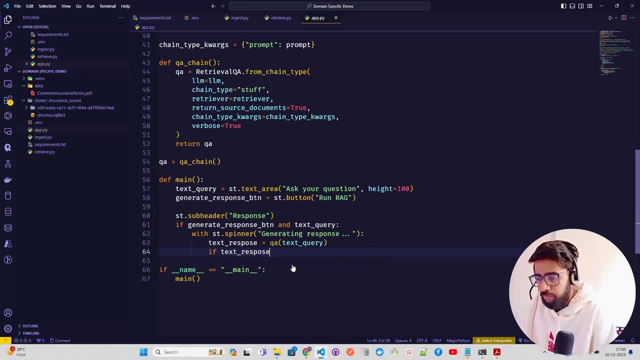 And then say, okay, if text response, ah, it's response. It's fine. 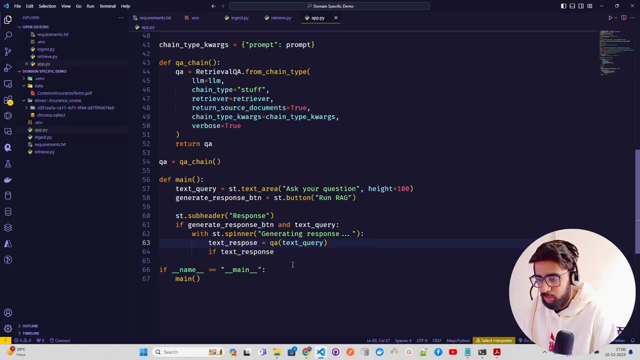 Okay. You can let me make the change, by the way, because you will be using the same GitHub repository, right? 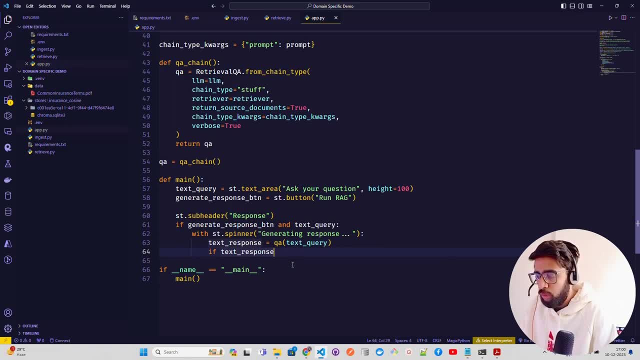 So if text response is HD dot right, and I'm going to do text response, HD dot success. 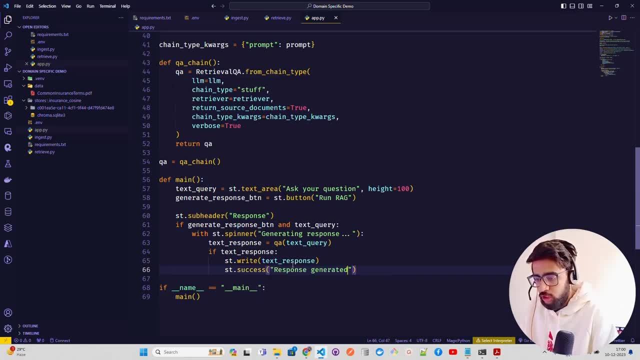 And here I'm going to do response generated. And then if not, then just give an HD dot error that, hey, I'm not able to generate the response. And then if not, then just give an HD dot error that, hey, I'm not able to generate the response. Response not generated. We are done with this guys. Now let me show what we are doing here very quickly. 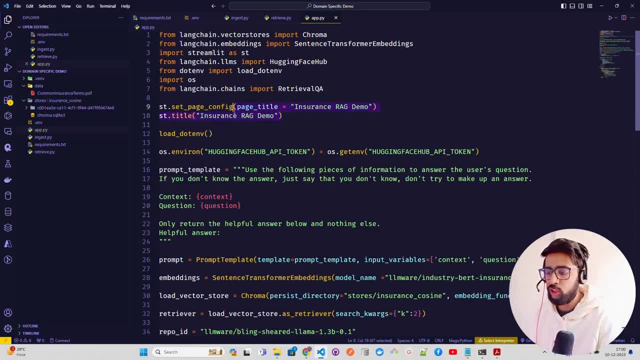 We have imported all the libraries. We are using extremely, so setting the page config, et cetera, loading the ENVs, you know, from, ah, that ENV file. 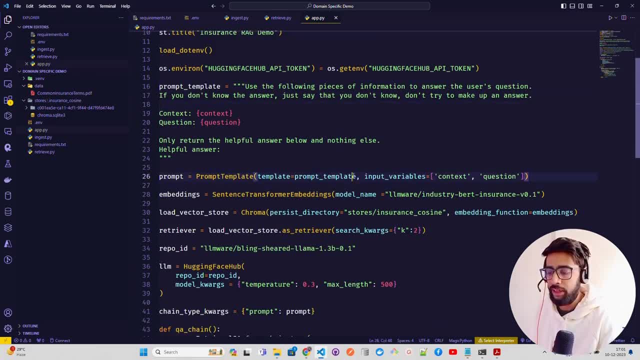 Then I have a prompt template. I have a prompt where I use prompt template, define the input variables, couple of variables. 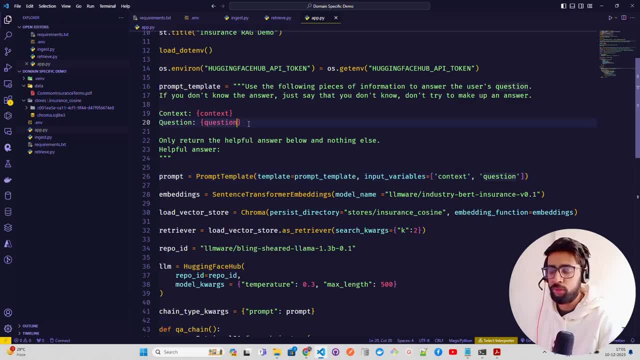 One is your context that comes from the retriever part of it from the vector database. 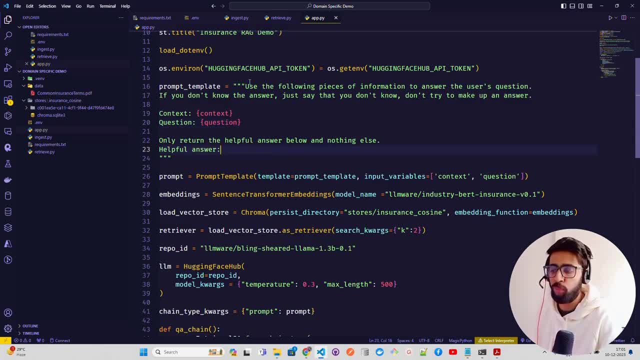 And the other is your question that the user will ask both gets combined with your prompt, and then it goes to a large line. This model to generate a human-like response. That's what it does. 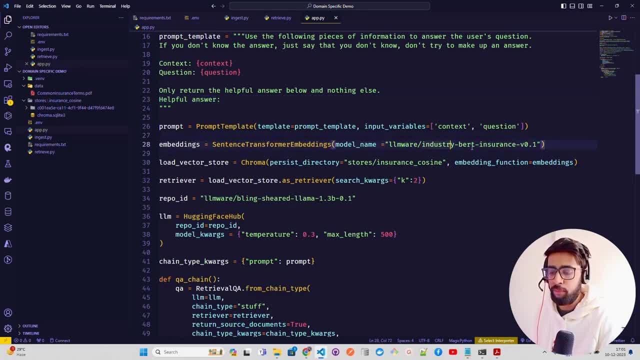 Now you have your embeddings where using LM, we are embedding, but insurance, then load vector store chroma from persist. We are loading it now. 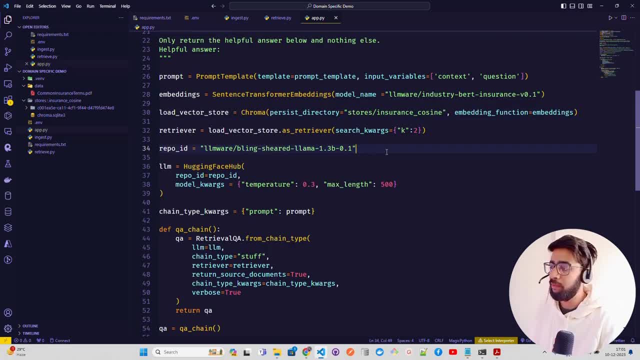 Then we are having a retriever thingy as a retriever search quacks, blah, blah, blah. And then we are just using an LLM that you can see from hugging face inference API, the seared llama blink where no GPU is required. 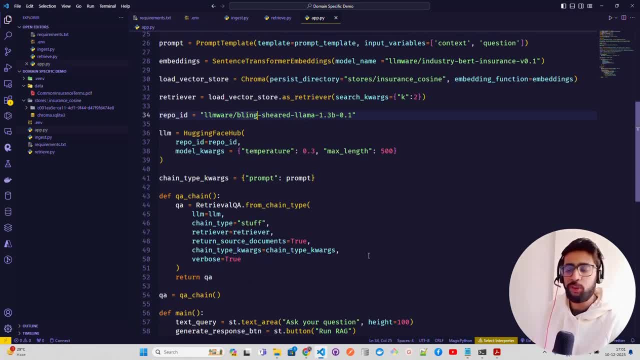 You can also download the model locally and do it through transformers pipeline. I think you can do that. 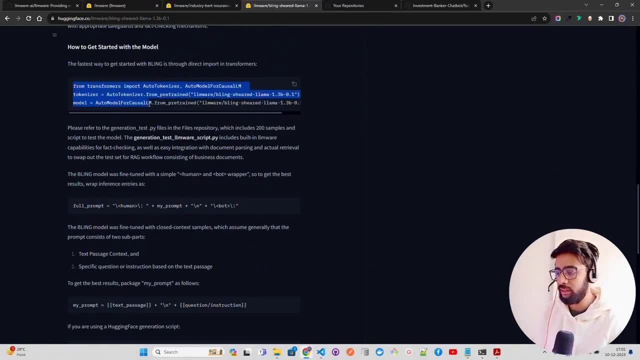 Much right, which is, which is so on here as well. You know, they have given some code. You can look at here, how you can use this code. Okay. This is our detail. 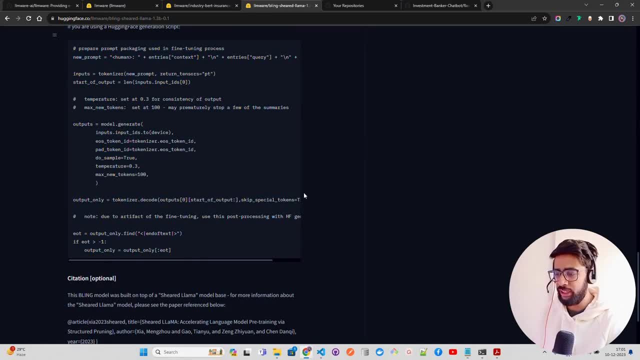 You can use transform a pipeline to do that, right? Auto causal LM. You can use it to do that, et cetera, because it's a text generation task. 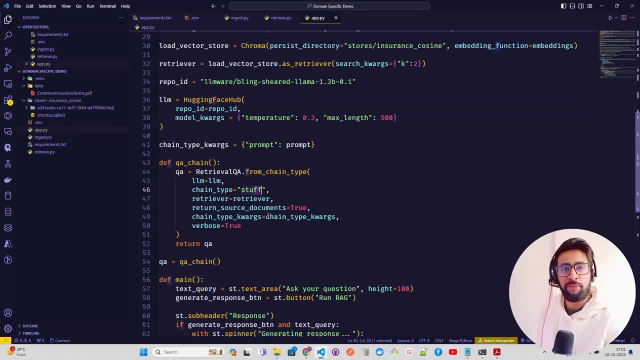 Now you have your QA chain retrieval, QA chain type, you know, defining stuff, uh, QA, blah, blah, blah, you know, extremely kind of thing to run that. Let's do it. Okay. 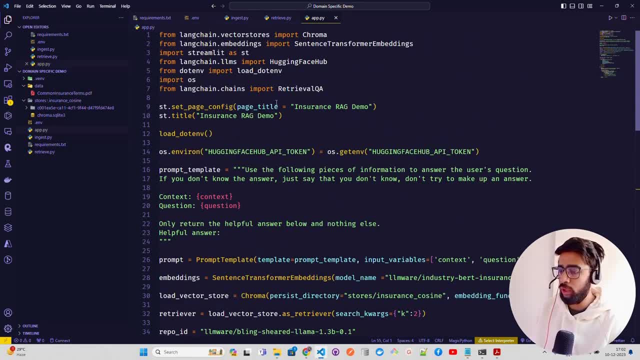 Let me see if we have imported everything. We have chroma. We have, you know, OAS retrieval prompt template. We do not have a prompt template. So let's get that. 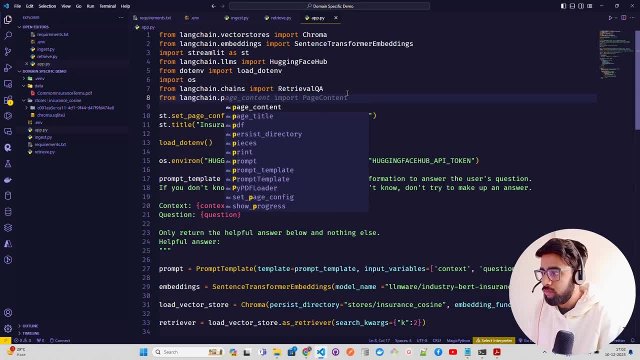 So from Langchain dot prompt, uh, it's prompts from Langchain dot prompt import prompt template. So this is what the prompt template is. 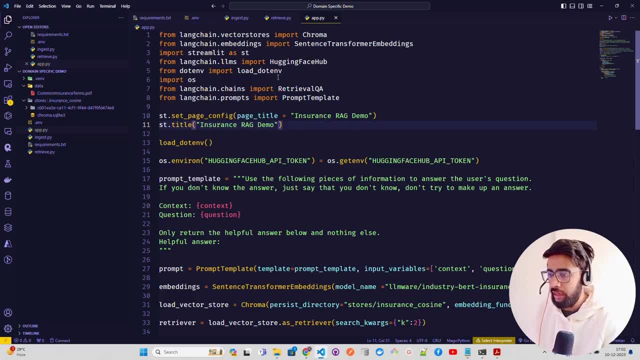 We have our sentence transformer embedding, hugging face, retrieval QA. Uh, we have chroma. Let's run it now and see if we get any error. 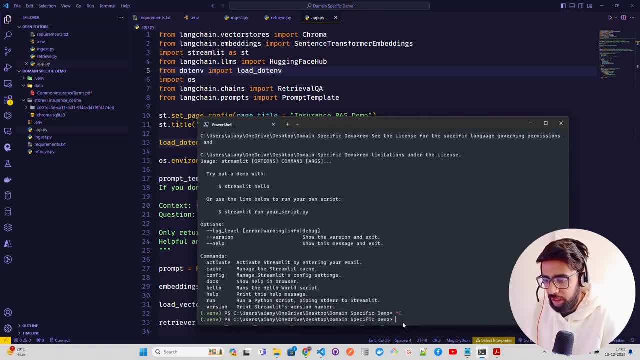 Now, what I'm going to do is extremely run, ah, extremely CMD by the way. Sorry. 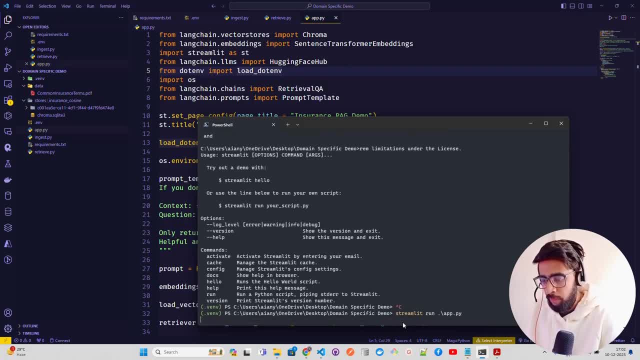 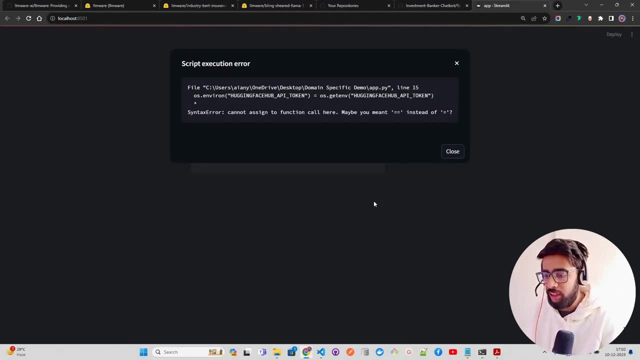 Extremely run app. This is. Once I do extremely run app dot PI, you can see what it says. It says, Oh, cannot assign to function call here. Maybe you want me. 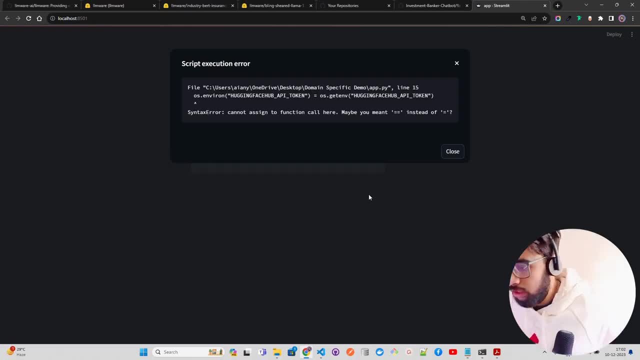 Okay. This is instead of this, this is okay. 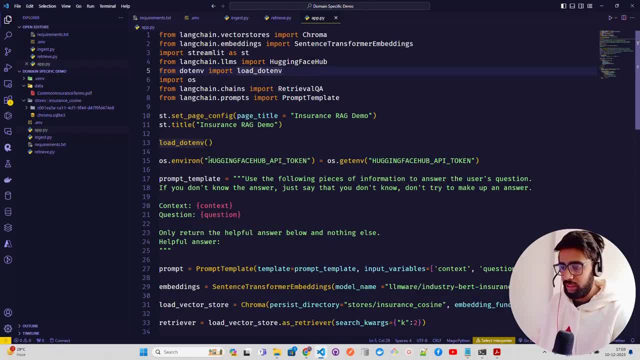 You can tell me what are the, uh, mistakes I have done here. It's not, it's not a method, right? This is my bag. This is my bag. This is my bag. This part is not a thing. 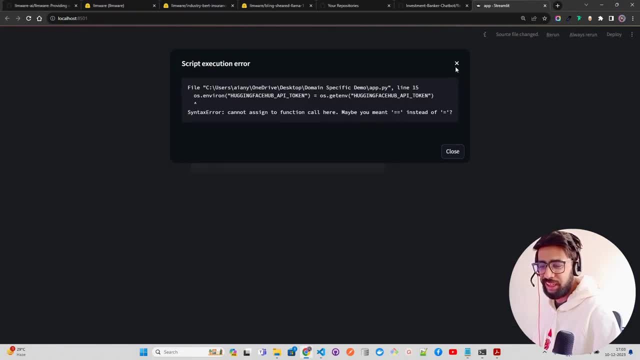 Um, which is. Uh, right now it's loaded. Let me just close this man. Okay. 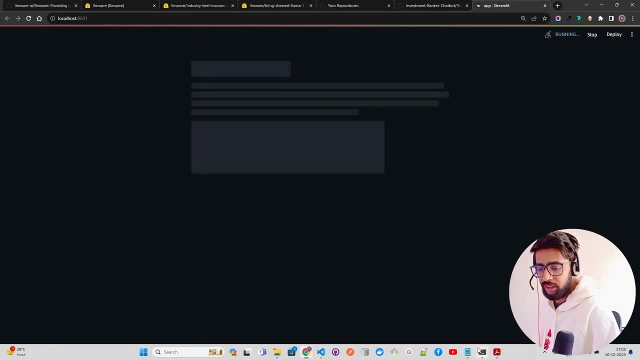 Uh, let's do a, can I do a rerun kind of a thing? Let me see. It's gives you something. I don't know if there's, there's still some errors. We'll see it out. Uh, for the first time, it will take a bit of time. Let's use the same question quickly. 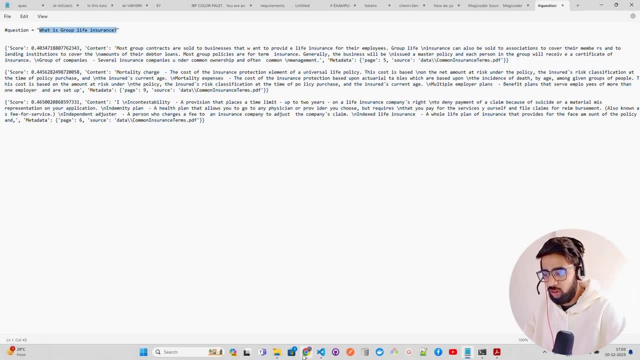 Uh, and we can also ask one more question and see if it's working fine or not. Let's use that here. Run rack. That kind of a thing. 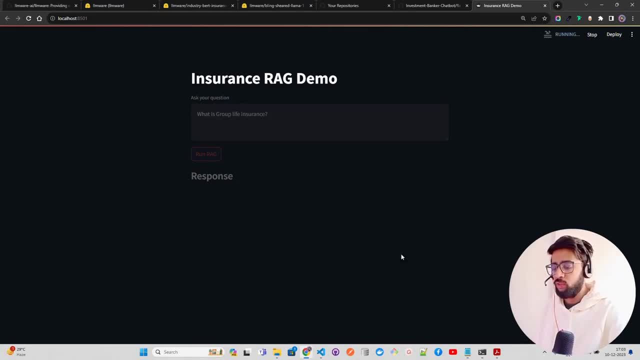 Once I do it, uh, you can see it's going to generate some response for you. 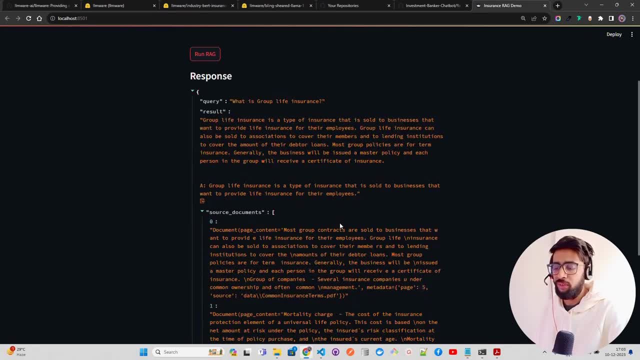 Okay. You can see it says generating response and fantastic, right? Uh, we are using, uh, LM. We are embedding model and, uh, LLM. And we get the output here. 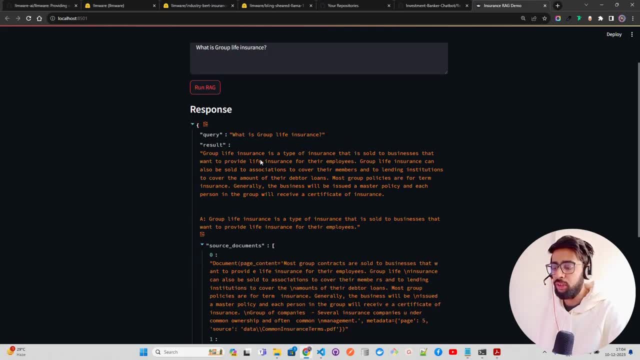 Queries. What is group life insurance? And it gives you a group life insurance is a type of insurance that is sold to businesses that want to provide a life insurance for their employees. 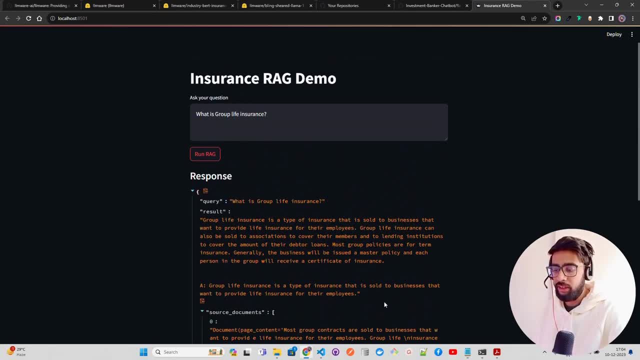 Fantastic. Uh, this is great. I loved it. Love the response. Let me ask one more question. 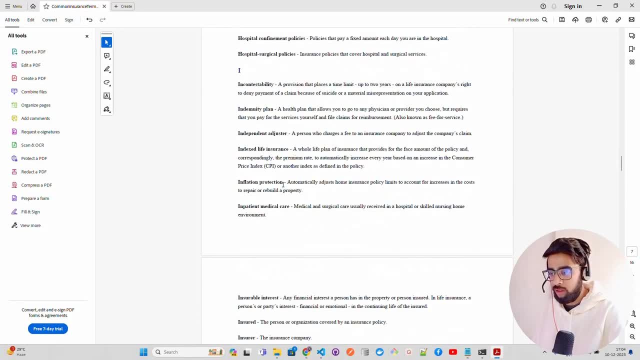 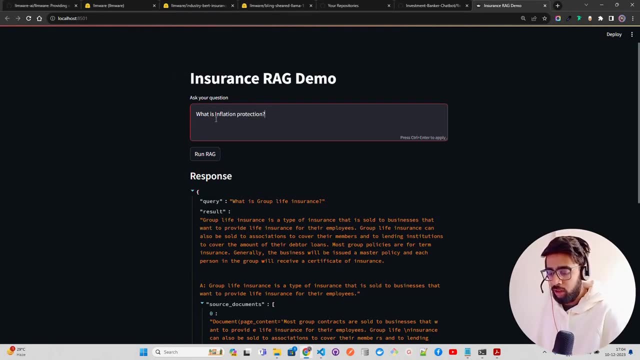 Quickly, what kind of question we can ask, uh, what is inflate inflation protection? Okay. Let me ask this question quickly. What is the inflation protection and see if it's able to generate some response and you can try it out, uh, for the complex use cases where you see there are chances of hallucinations. 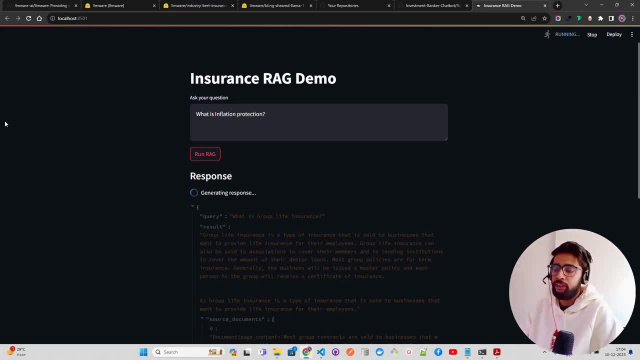 You can try it out. This model, I also wanted to test this model and in the first go on a very initial experimentation, I liked the model and the embedding model, both, you know, which is very lightweight. Okay. It's very easy to work with, very easy to deploy as well. Right. 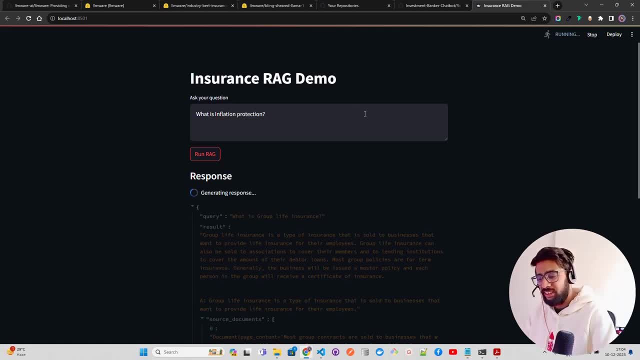 So let's try it out and see, uh, and it lets you generate, uh, the, the code is available on my GitHub repository. You can find it out over here. LLM where rack demo app. 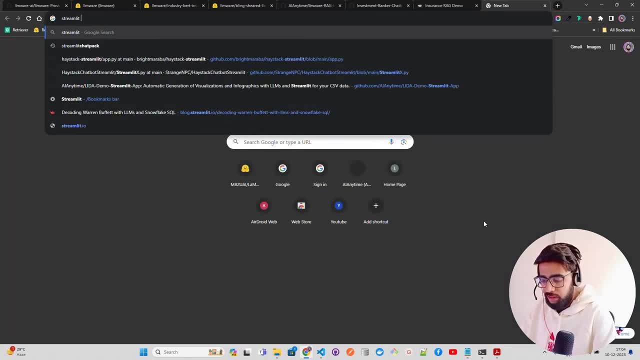 Let me just do one thing. Uh, I'll open a streamlit cloud or something like that. Okay. Extremely cloud. Okay. Let's see. 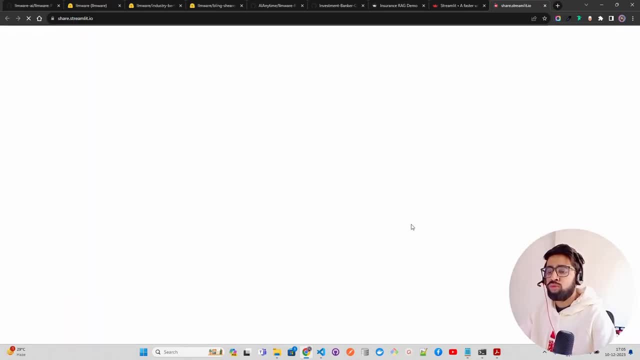 Sign in. So slow. Okay. Hmm. Continue with GitHub. 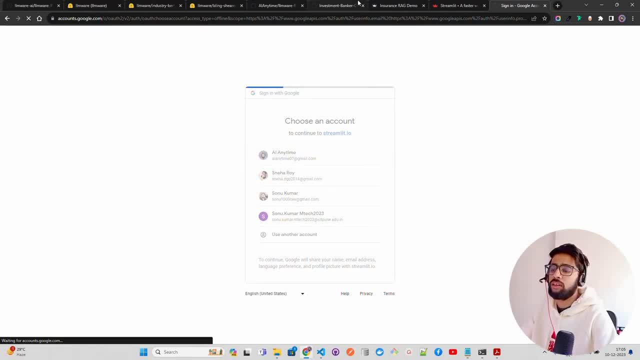 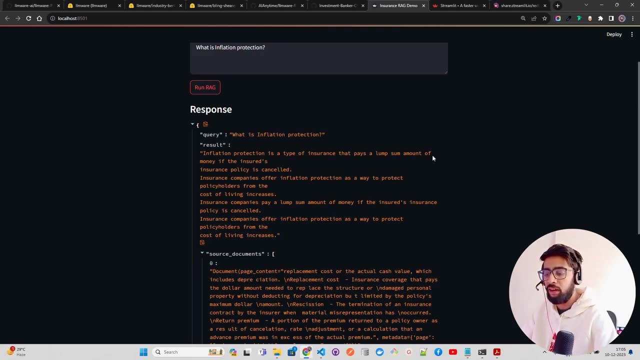 There is streamlit is something that where, you know, you can, uh, deploy your, uh, and you can see, we got inflation protection as well. So inflation protection is a type of insulin that pays a lump sum account, lump sum amount of money. 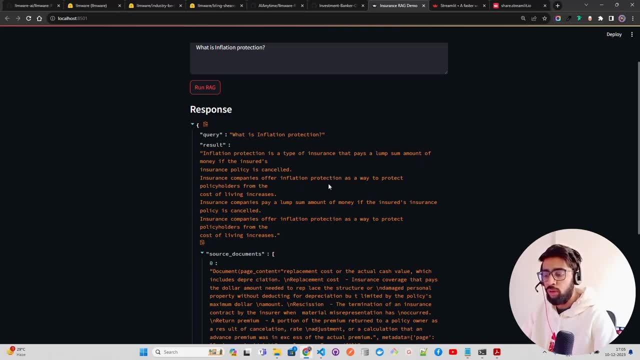 If the insured insurance policy is canceled, insurance company offer, wow, this is fantastic. 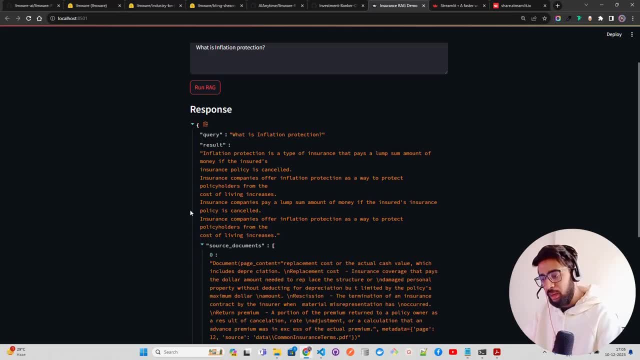 Great response from 1.3 billion model. I really loved it. 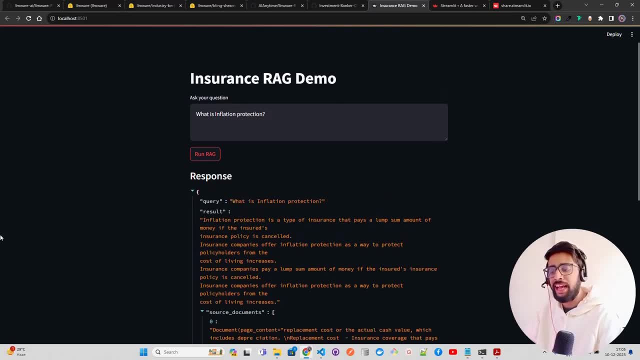 I think the credit goes to LLM where, and the AI blocks team, the more than happy to, you know, see that the future LLMs and the models that they're going to build. Now I'm going to create a new app. Uh, let me see that. 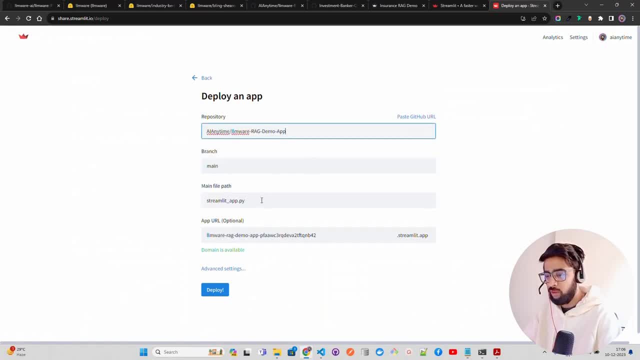 Um, let me see if I'm able to get something. 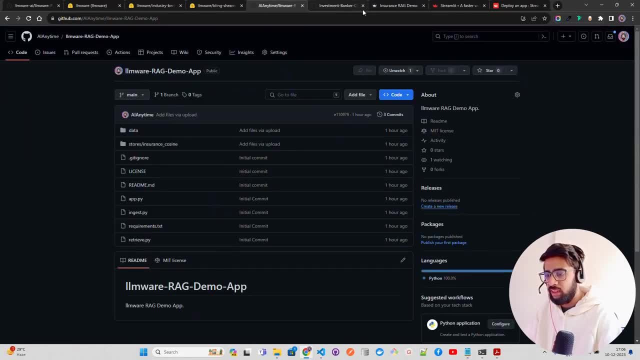 Okay. What is this file name? Where's this file? Okay. 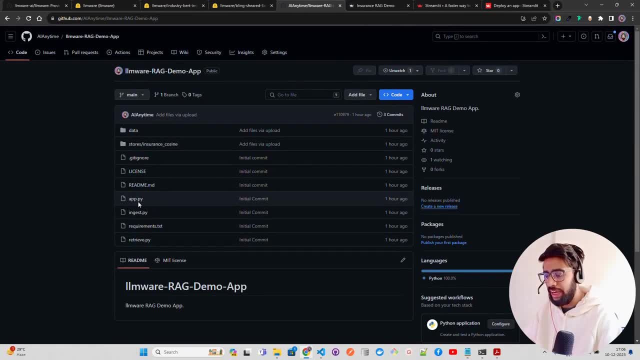 It's I've imported everything, right? The ENV is not there, but it's fine. So we have app dot PI. 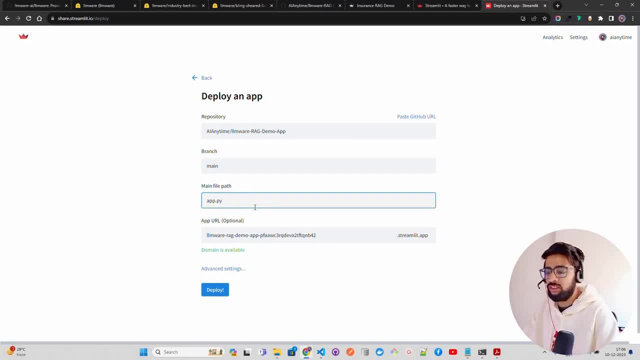 I'll just show you probably, I'll just not. So everything, but you know, this is how you can deploy. 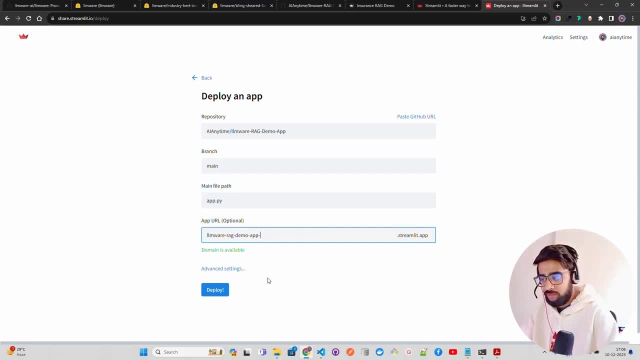 If you have an extreme lit app domain is available in the advanced setting, you're going to have your secrets. 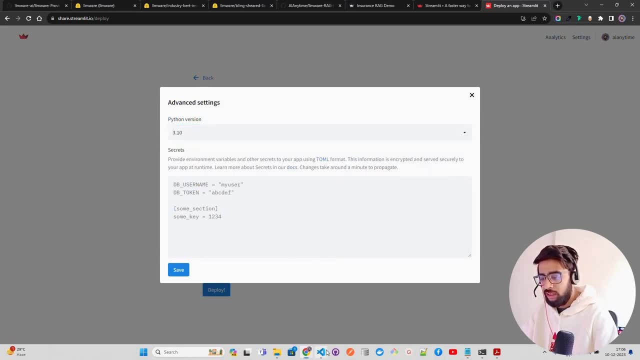 Let me use Python 3.10. And let me use this from ENV. Okay. 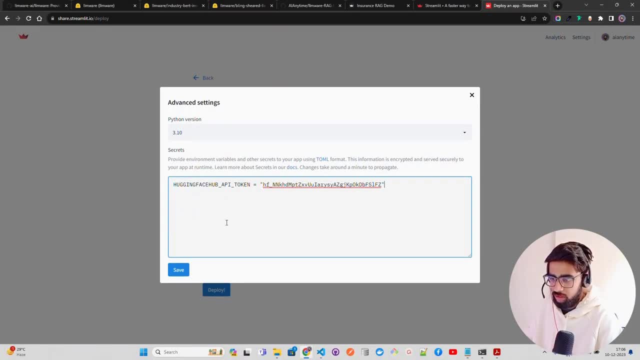 I'll just try it out. If this works, otherwise you have to see it. Okay. Save deploy. 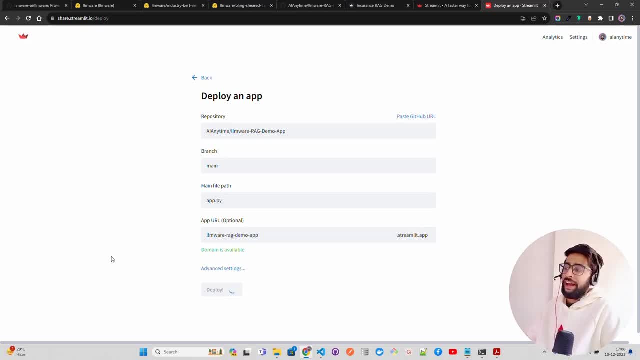 Maybe some requirements also we have to add, but this is how you can deploy an app. Okay. It gives you one GB free space to deploy. 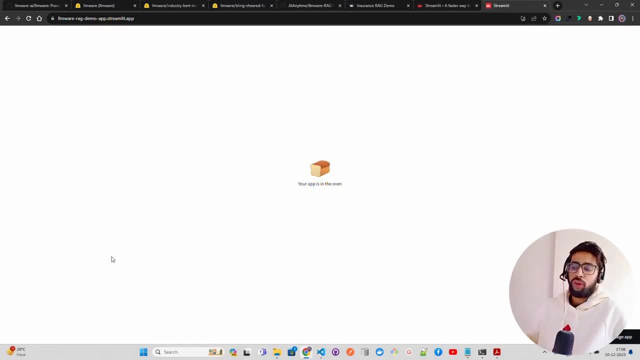 So if your entire folder is not bigger than one GB, of course, LLM saving locally will not help you to deploy like this on free streamlit cloud, but I'm using inference API. So I probably, I think I'll be able to deploy it. 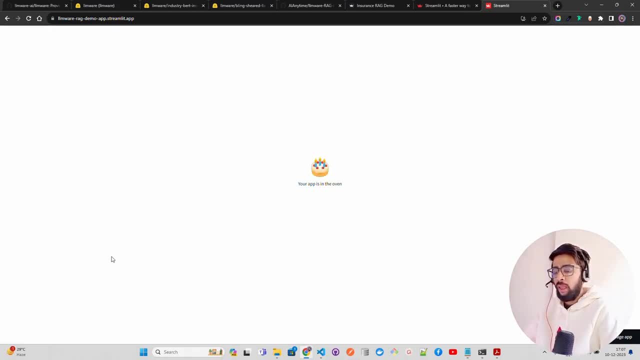 I'm not sure. Let's let's check it out and see if that that's a case, but if not, then you just got. The idea, right? 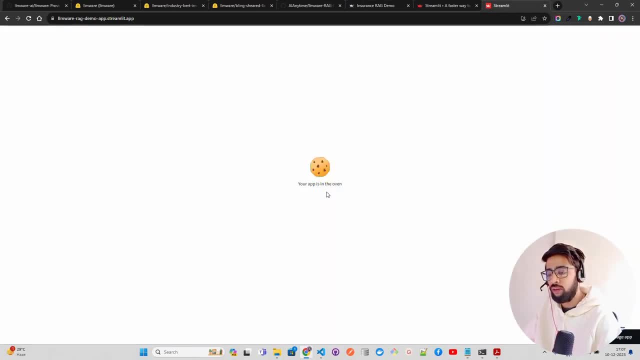 How to deploy. I think you'll see the app is working fine, you know, and you can find out the deployment over here. You can see it says, click on manage app, no installing everything. 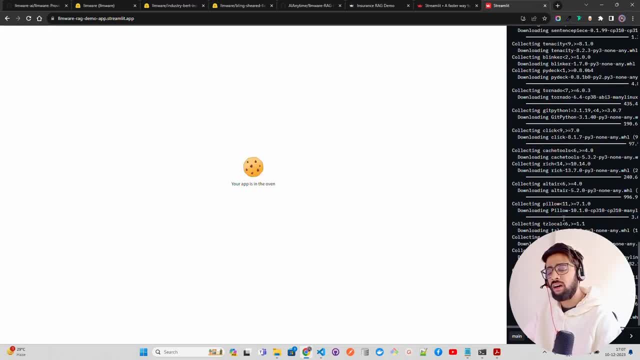 The problem is that you have to do a bit of, uh, work around here because for example, you know, you just saw NVIDIA and CC and all of those things have been installed. And I think we don't need it. So we should have just said torch CPU. 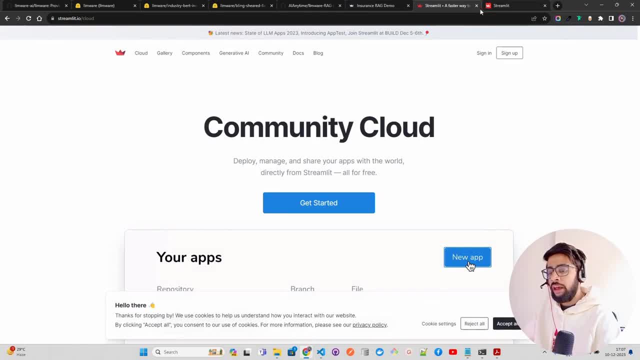 So it would only have installed or CPU, but it is fine. Anyway, uh, you can deploy your estimate app here. 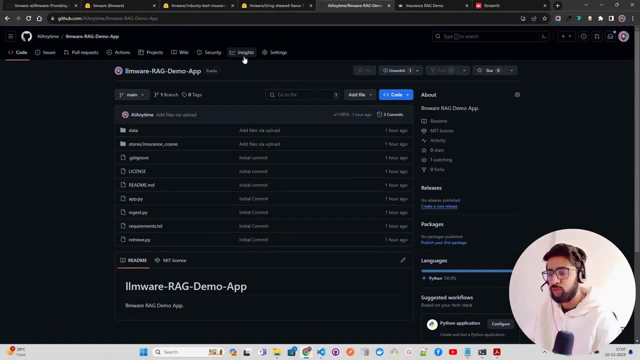 Incidents rack. Find it. See GitHub repository here. I'll give the link in description. 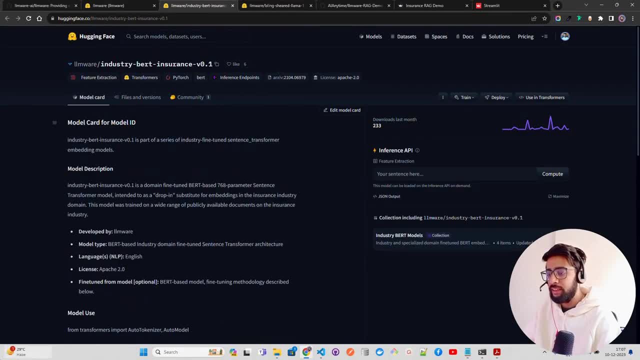 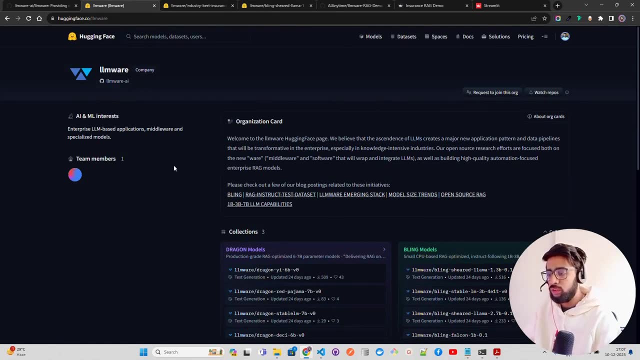 Find the models here by LLM, where find the embedding model here by LLM, where, and this is, this is the hugging face repository of LLM. Where, okay. So this is fantastic GitHub repo and that's all I can see. It says installing successfully uninstalled. Let's see. Let's see. 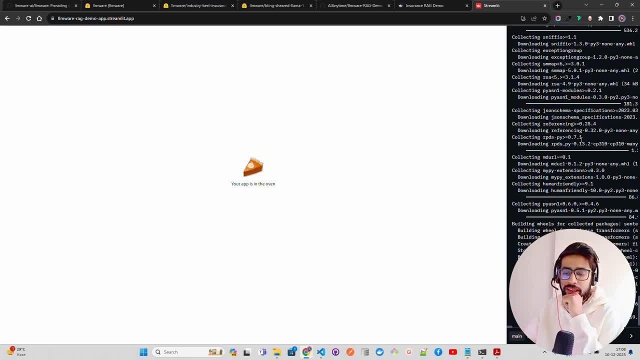 Let's wait for a few couple of minutes and see if it's able to deploy it because I, I believe that will exceed more than one. Uh, one GB of space because the embedding model is around 400 MBs of size, and then you have your, all the required dependencies that will again be around, I don't know, four, 500 MBs again, because you have torch, you have sentence transformers, NVIDIA, you can install something is not required, but, uh, let's see it out one more minute. And. Um. 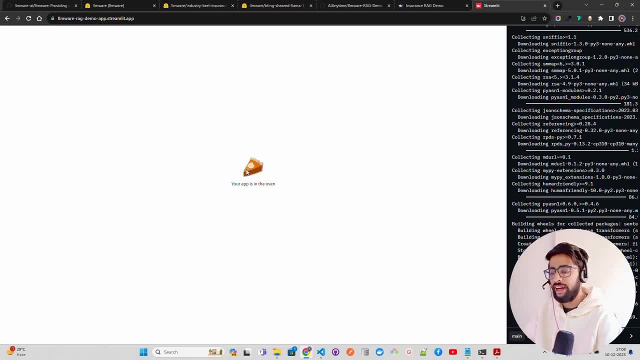 What you can see, it says your app is in the oven, right? I, I love the UX part of it. 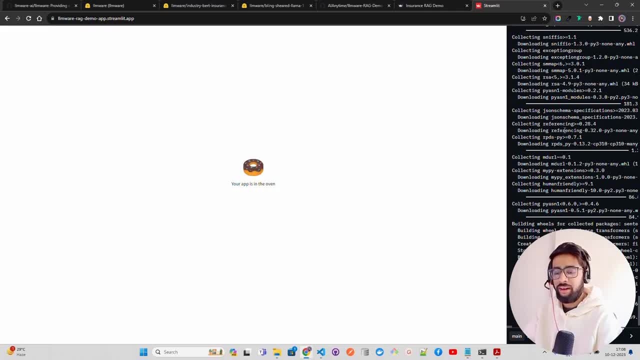 Uh, they will be using some socket programming to get the, uh, status from this part of it. That if that gets done, it will load the app. It's a containerized application. They use container to run this, but anyway, it's taking a bit of time guys. 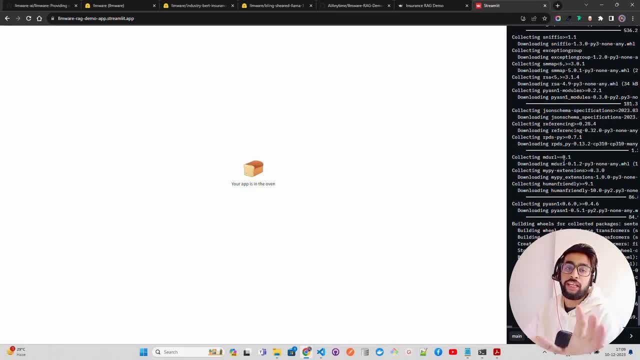 You know, if it gets successful, I will give the link in YouTube description and if it's not, I will not give it. So please excuse me for that. 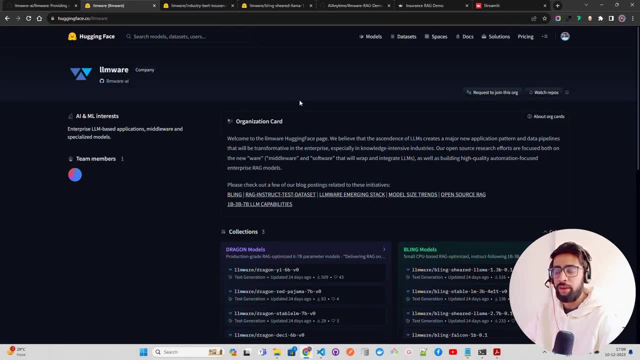 But this is the video is one more towards covering LLM where models and emitting models, because few of you also requested it. I, I could see. The comments and I hope you loved it. I liked it a lot. You can see the performance. Fantastic for chatbots. 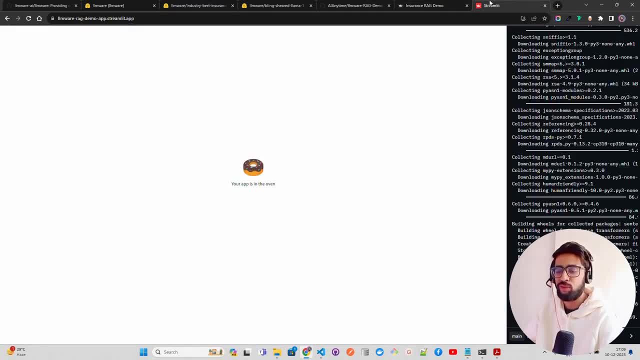 It's really good where you need probably not need a longer responses for that. It is good. 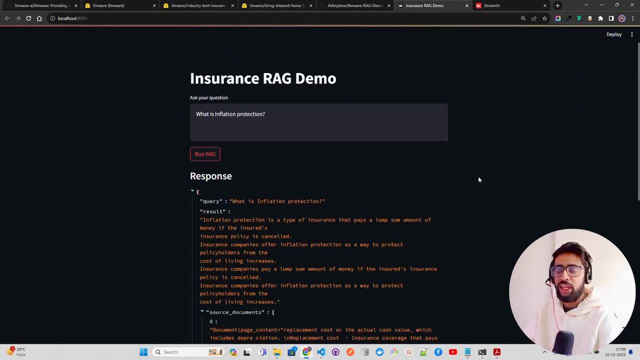 That's all for this video guys. You know, if you have any thoughts, comments, feedback, please let me know in the comment box. 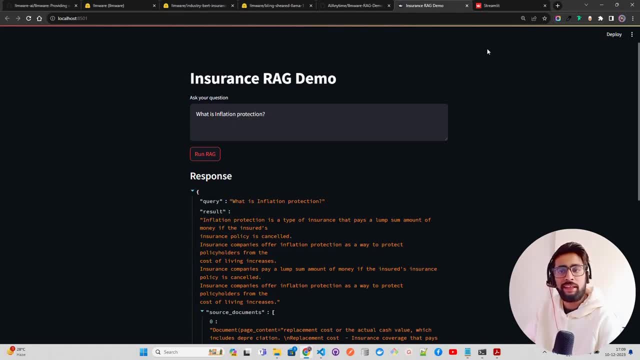 If you liked the video, please hit the like icon. If you like the content I'm creating, please share with your friends and to peer and also subscribe the channel. 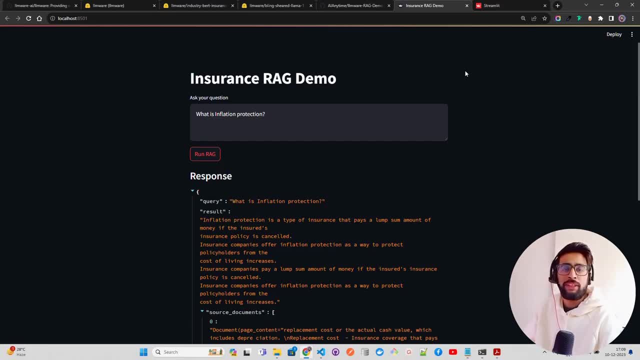 If you haven't subscribed the channel yet, thank you so much for watching. See you in the next one. Bye. 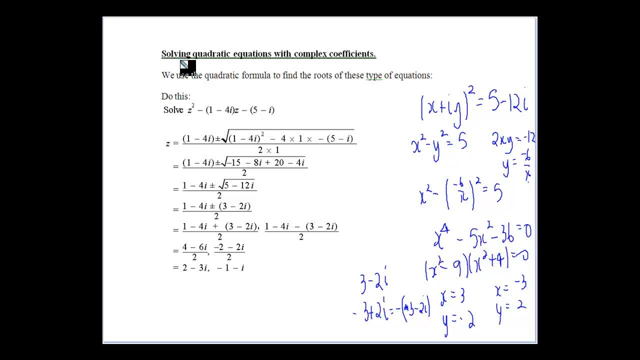 Okay, let's have a look at this problem here. This one's solving quadratic equations again, but this time we've got complex coefficients. We haven't got our nice real coefficients, So this starts to add a little bit extra difficulty to the problem. So, really, what we need to do is: 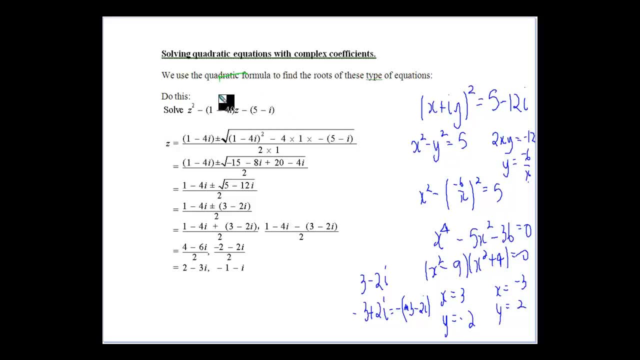 use quadratic formula. Forget about completing the square, definitely forget about factorization. We're going straight with the quadratic formula. So we've got minus one minus four i, so that becomes negative b, which becomes positive Plus or minus the square root. Okay, we've got the. 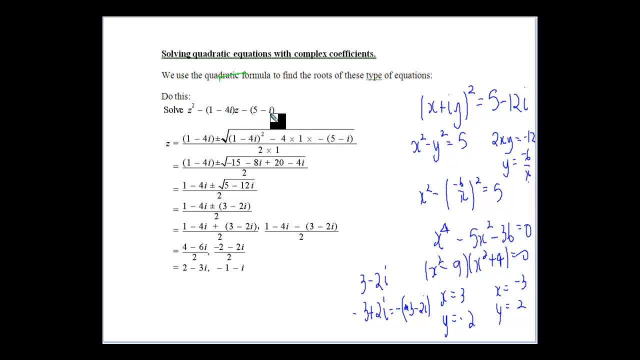 discriminant. there b squared minus four times a times c, So over the two times a. So expand that out. So multiply that out. Multiply the minus four times the minus five gives you plus 20.. Minus four times, minus four times. 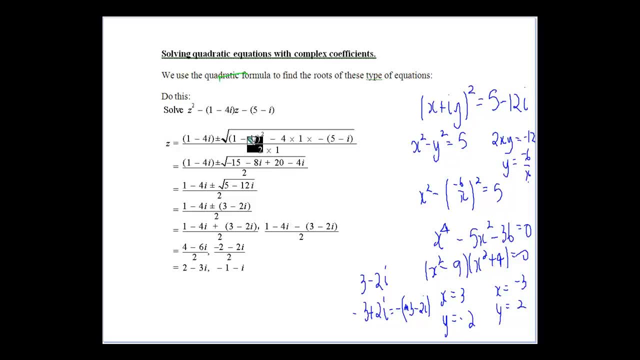 minus minus i gives you minus four. i Collect our terms. That's minus 15 minus eight i is the expansion of that. one Comes down now to this situation. We've got the square root of five minus 12 i Now. in our previous video we looked at how to find the square roots of a complex number.